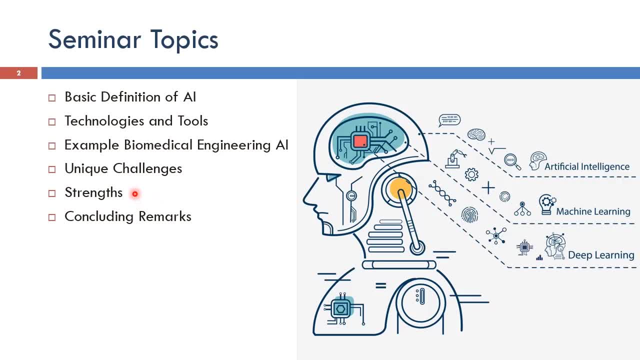 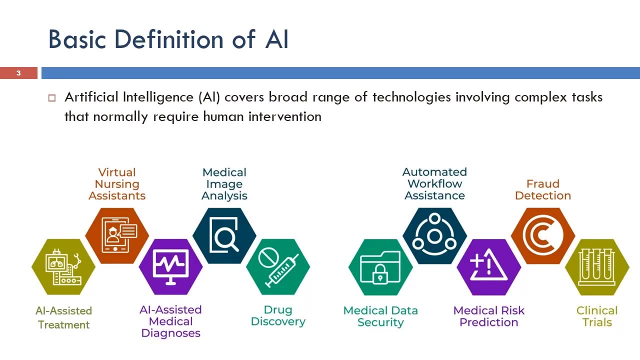 than the other areas. Then I'm going to just talk briefly about the potential strengths in using AI in biomedical engineering, and then I'm going to have some remarks about what we talked about in this talk. Artificial intelligence covers a broad band of technologies involving complex tasks that normally would require human intervention. 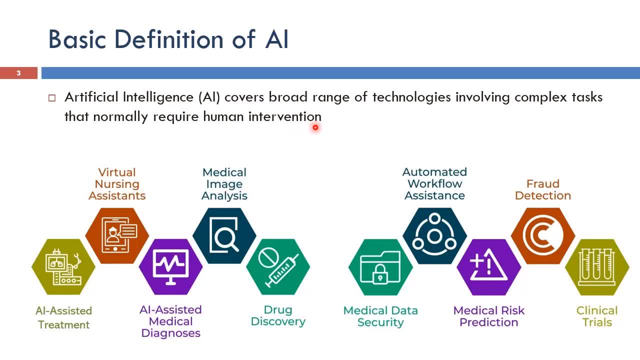 It has so many different applications in biomedical engineering, including basically medical image analysis, including drug discovery, AI, medical diagnosis. It has some other managerial things like a nursing assistant, like basically, if you have medical data security, if you have medical risk prediction in like insurance companies, things of that sort, and also in 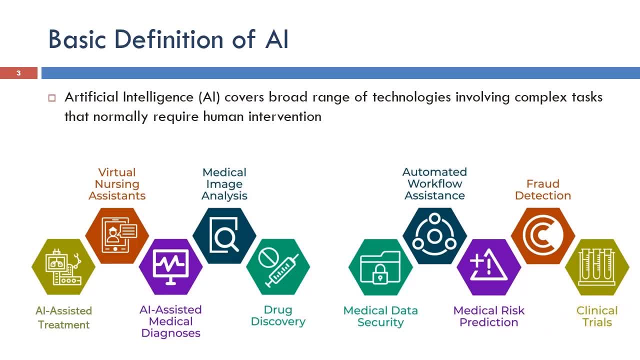 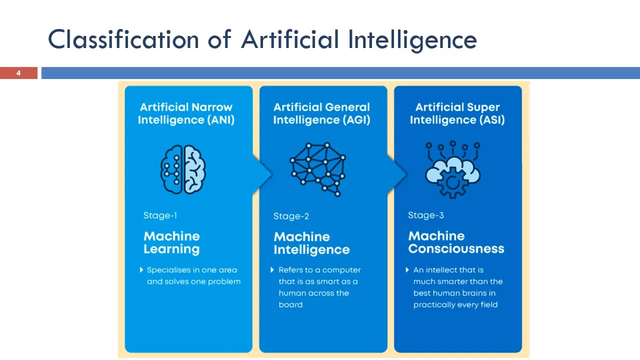 managing clinical trials. Basically, it has so many different applications, but we have to be sure that this technology is appropriate for each one of these technologies or each one of these applications. We can classify artificial intelligence into three main areas, or basically three main stages. The first one is what's called the nullity. 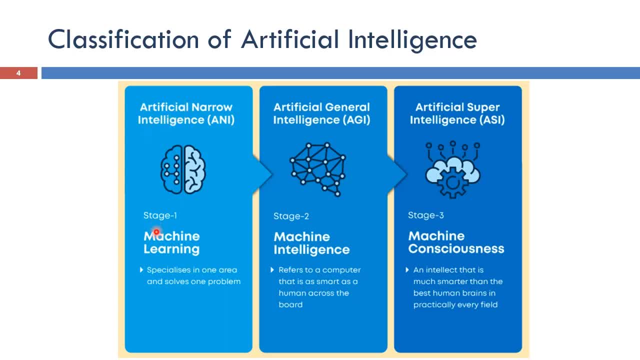 Nullity is a narrow intelligence or narrow artificial intelligence. Basically it's mainly, you know, concerned with machine learning. Basically, it's an artificial intelligence system that specializes in one area and solves one very particular problem. Basically, most of the AI systems we have right now belong to this stage. here There was like an ambition for the technology. 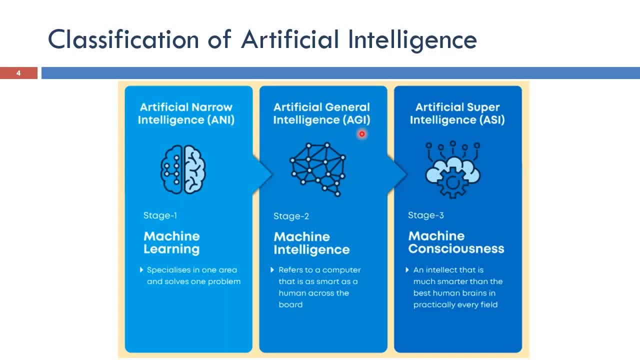 to become artificial general intelligence. Basically, this is the artificial intelligence system that would act like a human being, Like basically it can learn new things, basically on its own. It can. basically you can start with a very specific application, but actually it can generalize the application. It can learn as very. 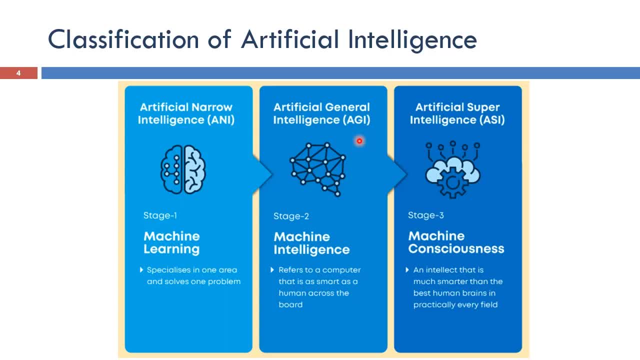 much as a human being. This is a little bit theoretical right now and we are very far away from it at this point. The third stage is even beyond that which is called artificial super intelligence, In this case actually talking about machine consciousness. Basically, you're talking about 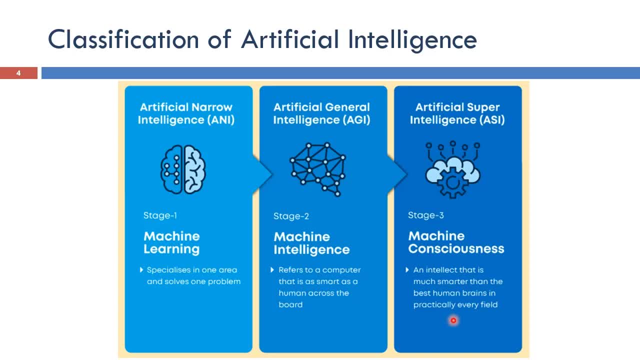 a machine that knows about itself, Okay, like that can basically have a similar consciousness as a human being. This is kind of in the realm of science fiction right now, because basically, or it's maybe technology for science, but I suppose it's in the realm of the airports, being kind of. 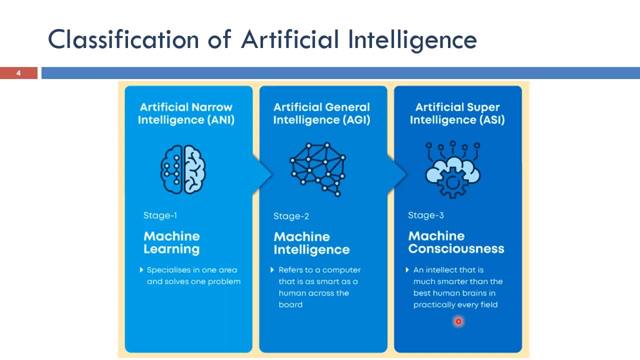 awesome. So let's talk a little bit to that state and kind of where that contenido goes. I think communication science is still in its early stages, where all the machines are Eine feeling like a machine goal from what we are, what, what we have right now one major problem of 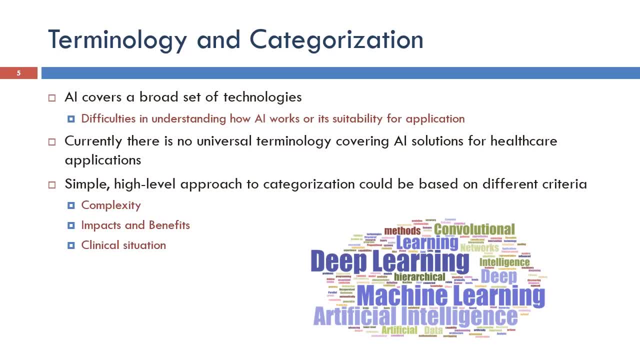 artificial intelligence in that it has a problem in terminology. okay, we said before that the AI covers a broad set of technologies. basically, you you hear about different terminologies that are used like, for example, deep learning, machine learning, artificial intelligence, convolution, neural networks, single, that sort, and basically, which one means what? okay, this is a big problem currently. 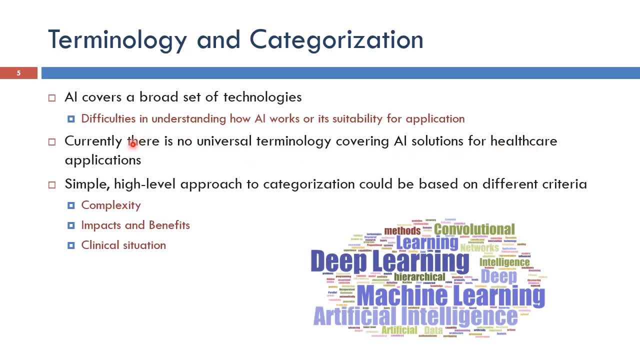 there is no universal terminology covering AI solutions for healthcare applications in particular. okay, but actually we can suggest that it might basically be developed based on simple and high-level approach to categorization that could be used in different areas, basically different criteria like complexity, like impact and benefits, like clinical situation. but 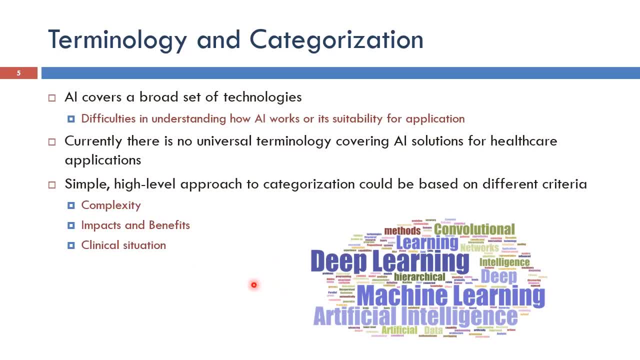 if you, if you're talking about a particular AI system, it's sometimes very difficult to basically understand what what the person is talking about, because sometimes, when you talk about artificial intelligence, you would mean something that is very basic, as regression, for example, and basic you can mean something. 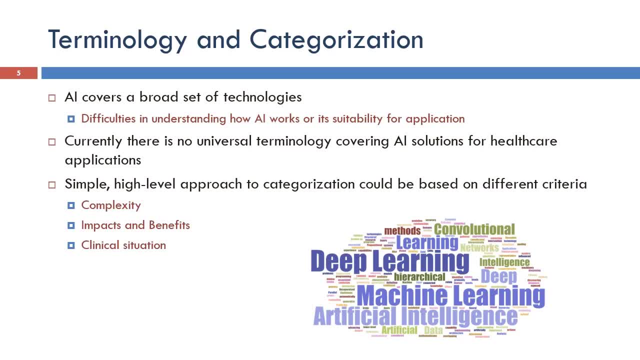 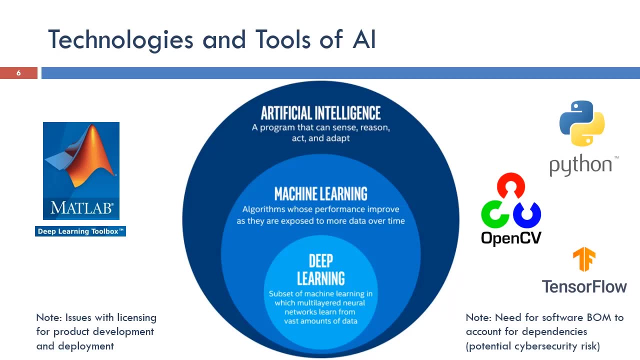 that is very complex, like deep learning. so basically we have to start thinking about how to standardize the terminologies and the categorization of the technologies involved in AI, particularly for medical applications. in general, people basically consider artificial and intelligence as the umbrella for all the technologies that are involved. that basically involves: 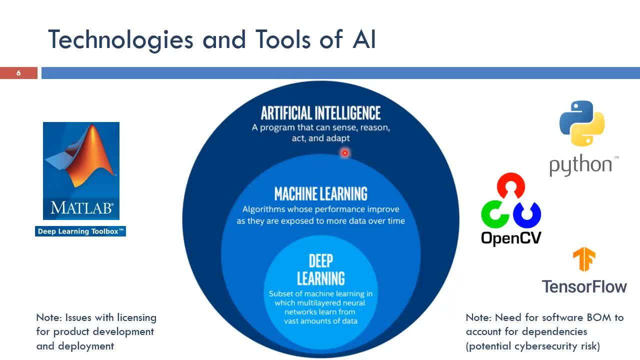 programs that can sense, reason, act and adapt. okay, a sub categorization or subclass of artificial intelligence will be machine learning, which is basically a system that could be trained over time or trained on data so that it can actually improve over time. deep learning is a very special class of 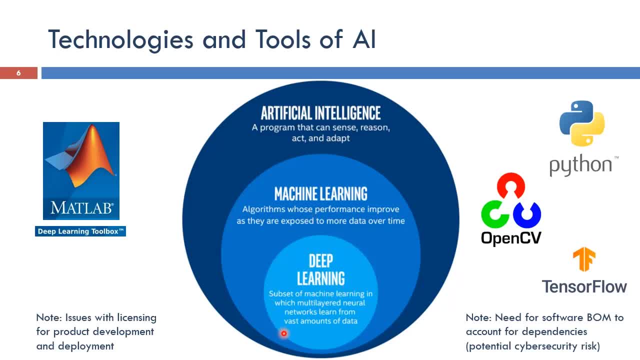 machine learning, which is based on very deep neural networks. we're going to talk about how this works in a second, but basically this is a subclass of machine learning. in order for us to be able to use artificial intelligence, we have to have tools, will have to have programing tools that that would allow us to do. 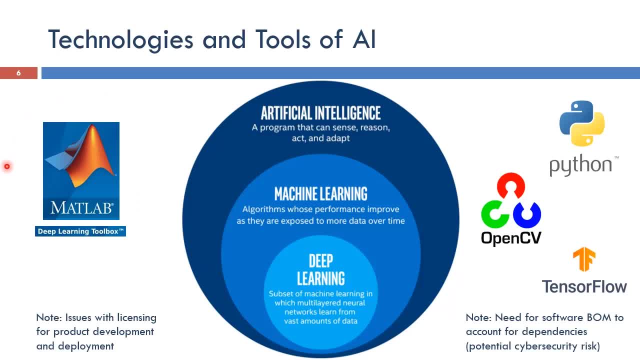 that okay. the on one side we have MATLAB- we have a deep learning tool based on a machine learning, and the other side we have an artificial intelligence tool based on a box. we have machine learning functions. we have so many things that we have in MATLAB, but the problem is we have to have licensing for MATLAB and we have to. 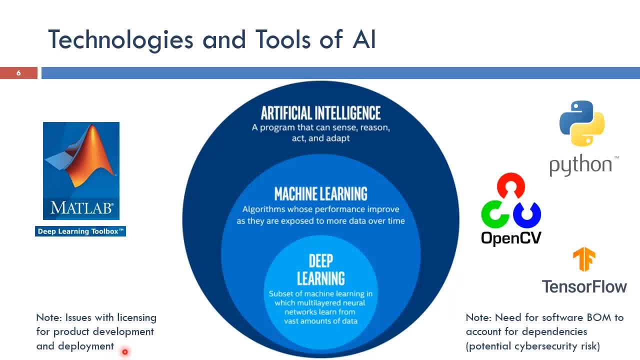 have it for product development and deployment. if you're going to deploy a product based on MATLAB, I think you would have to have a license and, by the way, the academic license is much cheaper than the industrial license. basically, if you're going to have a product with MATLAB, then you have to really think. 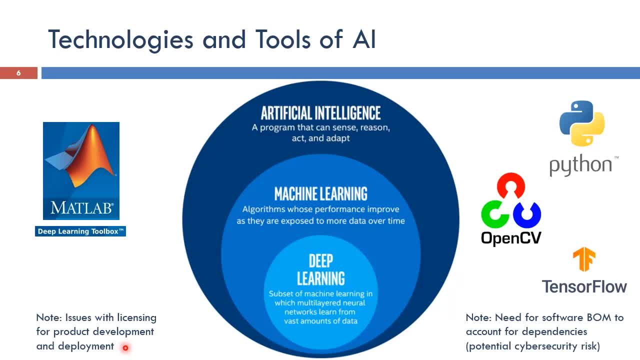 about how much you have to pay for having this software in your company. this is really gonna be a concern. on the other side, you have the open source community. you have Python, you have OpenCV, you have TensorFlow. you have a lot of tools actually, and most of the people working on research in AI they 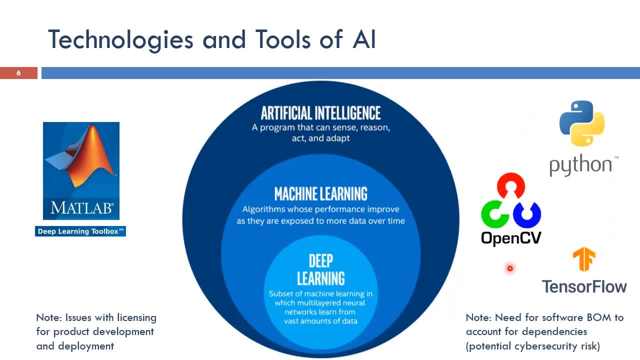 actually use the open source tools that are available from the open source community. okay, the problem with open source is that right now, the hackers are not waiting for softwares to come and basically find, find the bugs or find the exploits in these packages. they basically- they are basically involved in the open source community right now and 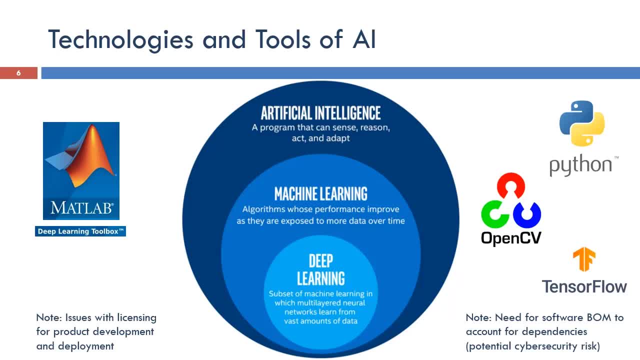 basically the inject, or basically put some code in each one of the or several of the very popular packages that are available for programming and basically, you would end up having a problem or a concern about the cyber security of your application. so this is a very big problem. in order to solve this problem, 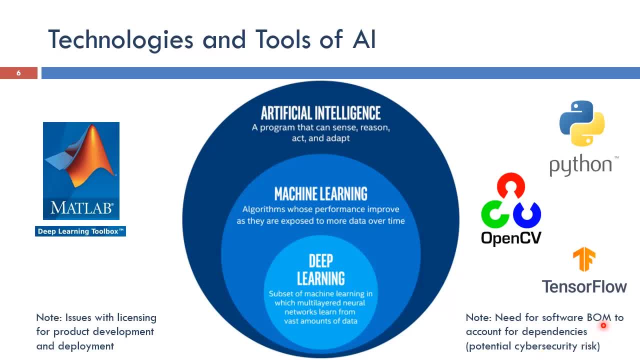 you have to have what's called software bill of material. software bill of material is basically a list of all the dependencies in your program, the open source program. so basically, whenever you use a package or basically use a package that uses another package, you have to actually list all of these so that when 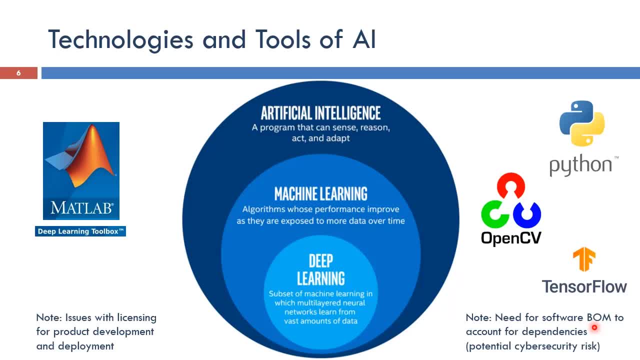 people discover a problem or an object in one of these packages, you would learn about that and fix it in your code. okay, so basically, this is definitely it's open source. it's for free. you can basically get started working on AI right away without you know basic. 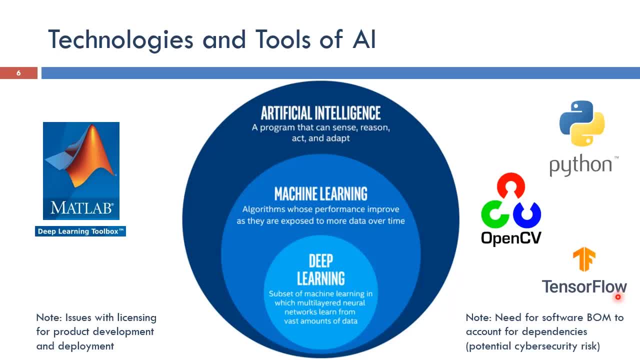 with minimal cost. you just have to have the computing hardware. but the problem would be in the potential cyber security risk. in addition, of course, as open source, basically you have no control or the versioning, for example for Python. if you have Python 2 or Python 1, you have differences between Python 2 and Python 1. basically. 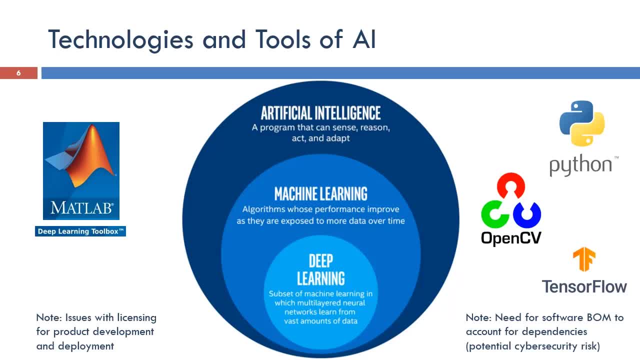 and basically some, some of the code might not be compatible. so basically you have to. whenever you start building a project, you have to stick with a particular version until you finish and then address the differences that might come in later versions one by one. you know after that, since most of the 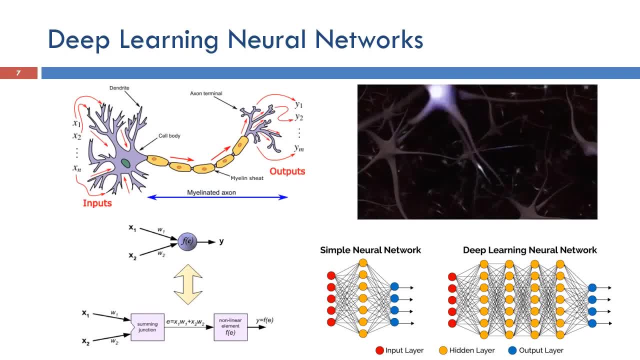 impressive results that came out, you know, and basically motivated people to use AI, came from deep learning. we're going to just give a brief idea about what deep learning is and how it is constructed. basically, the solutions based on deep learning are based on neural networks and neural networks. 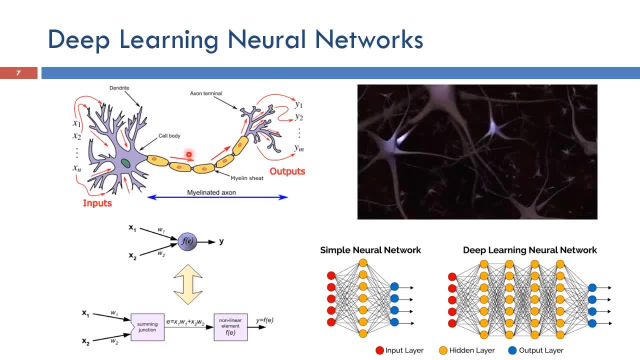 actually tries to emulate or simulate the actual neurons that are present in the brain. basically, in the brain you have billions of neurons that are interacting together, and together they actually do all the functions that we do in in the brain, which are basically, basically the edge cells of the brain. if we don't, 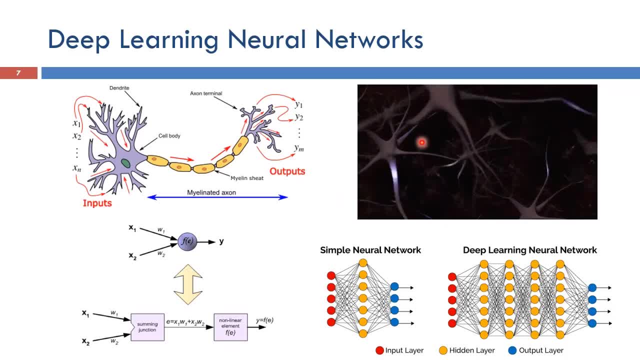 is the intelligence, the natural intelligence we have comes from the interaction between neurons. So people try to simulate the neurons. basically, the actual construction or action anatomy of a neuron is like a cell body and you have an axon and you have what's called, basically, terminals. 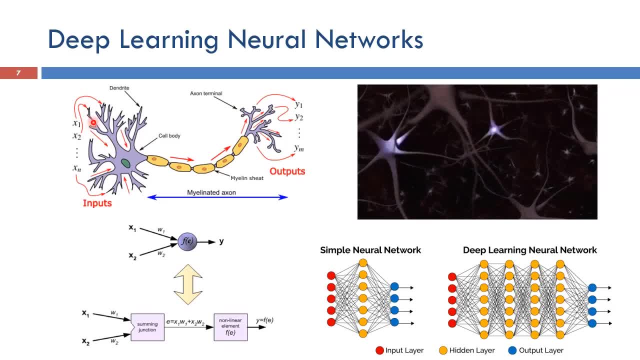 here. okay, You have here dendrites that would actually interface to action terminals from another neuron. So basically the signals comes from here and goes to the cell body where it's processed, and then it is sent on this cable. It's basically it's a myelinated axon. 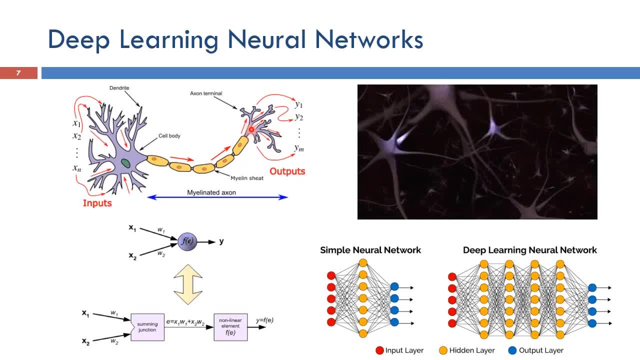 for example, basically where actual signal gets transmitted here and basically interface to another neuron through the axon terminal. So basically the idea is very simple. basically, If you want to simulate this, basically you have to have inputs And basically each one of these inputs might have a weight, because each one of these dendrites might 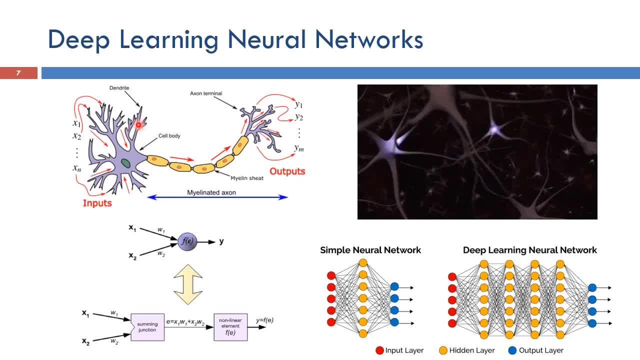 have a different path and basically it would basically weigh or put a weight on the input based on this path, for example, And then it goes into a processing unit here with a function that takes basically the inputs from here and applies a particular function on these inputs and produces 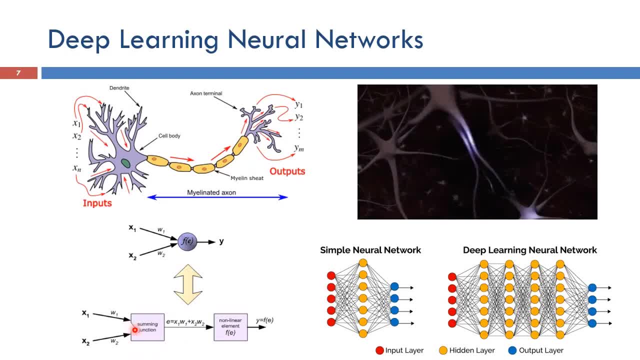 the output. If you want to make it a little bit simpler. basically there is a summing junction here Where you multiply the weight by the input. so you have w1- x1 and w2- x2 and just add them together. At this stage you have a linear system. Linear system cannot really produce something that. 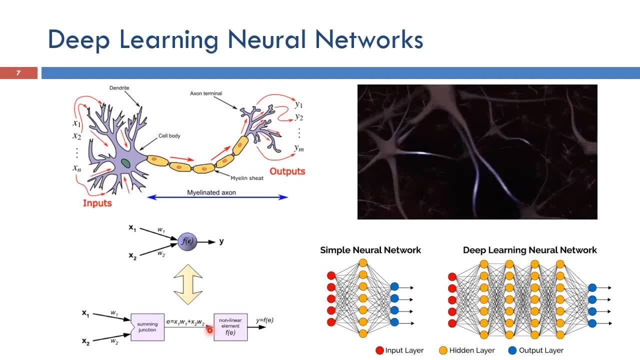 would be very useful because basically at the end, if you add several linear systems together, you will end up being one linear system. But actually if you add the nonlinearity here, if you add a nonlinearity, that looks like a sigmoid function, for example. 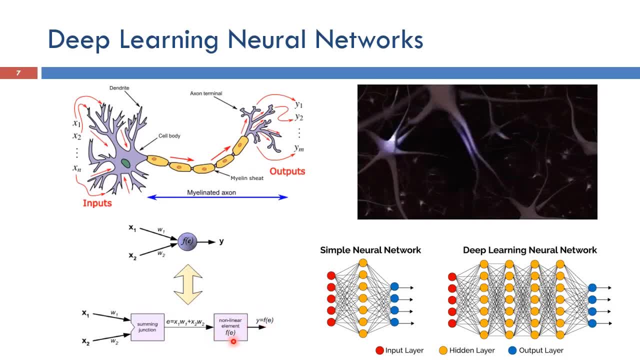 you will end up with something really useful. Okay, so basically, a nonlinearity here can be added, and non-linearity can be selected between several functions, including a sigmoid function, for example, and then the output is produced. newer networks started. uh, very simple, okay, they had. 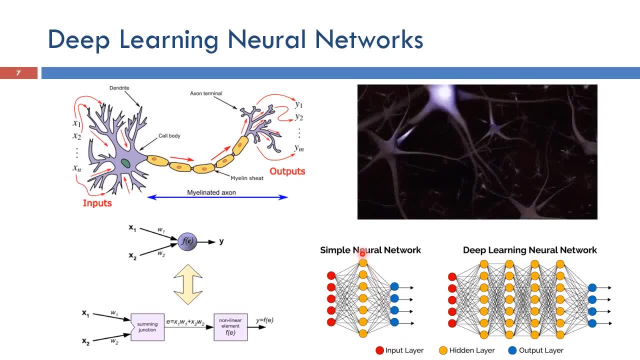 an input layer, an output layer and what's called a hidden layer. the hidden layer is basically whatever, uh, whatever is in between the input and the output, because basically, if you look at the neural network, you consider it as a black box. you don't really know what's going on inside. 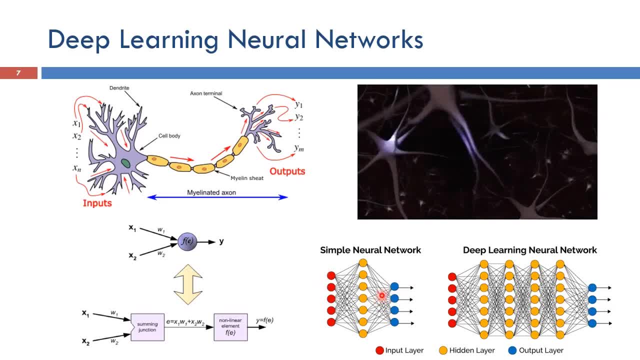 you see only the input side and the output side, so basically whatever is inside here is hidden and basically this very simple neural network was very useful and people used it for basically now we can say that more than 30 years now in classification of basic, basic, basic classification. 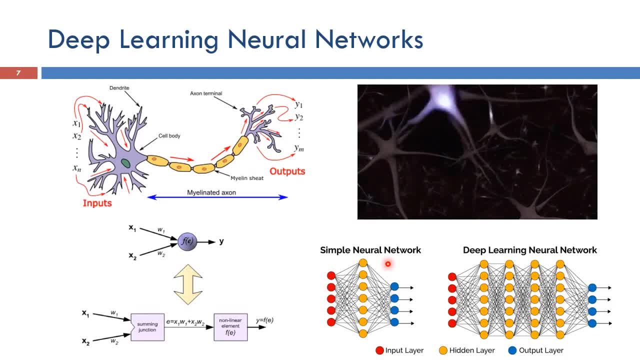 tasks in different areas, but the breakthrough came when people started putting a lot of- uh, basically a lot more hidden layers in between the input and the output. okay, so basically, if you have a deep learning neural network, you have so many different layers in between here and basically when you do that, you start seeing a lot of improvement in in the 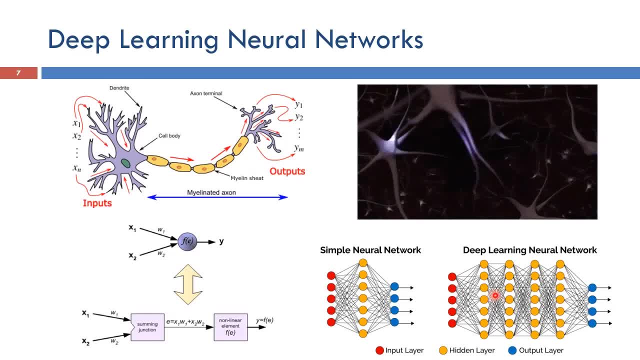 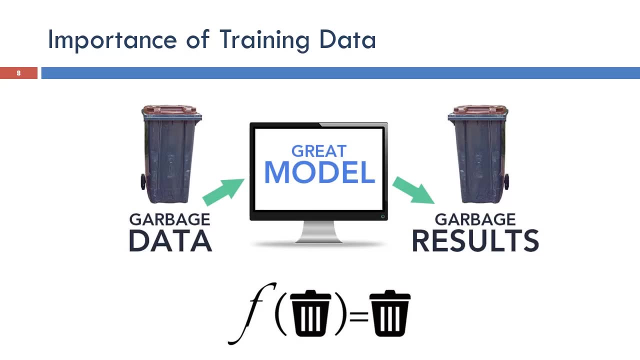 results okay and you can handle, uh, basically, very complicated classification problems and basically you start getting the impressive results that we see in different applications. so basically, we have a model. we actually the, the the deep neural network model is already there. people know it okay. why isn't it working for everything? 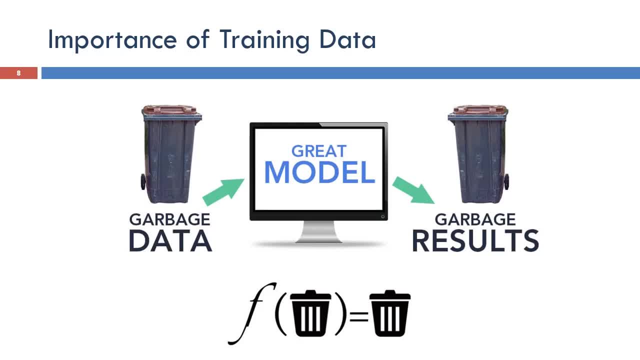 basically, the the main thing about any model is that you have to have great data. you have to have really good data in order for this model to be trained properly, in order for it to basically be useful later on. so basically, if you have the greatest model in the world and you 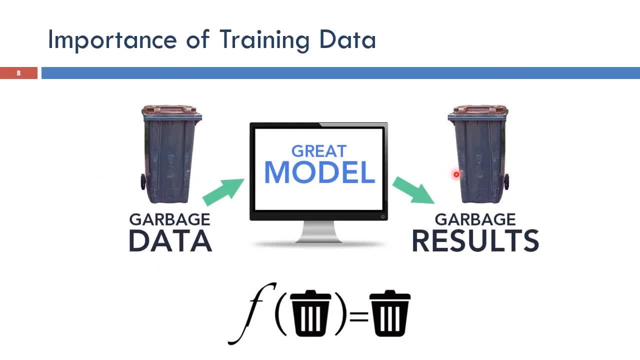 it or train it using garbage data, you would expect to have garbage results, okay. so basically, this is a very big problem in all areas. basically, you have to make sure that whatever you have for your data in order to train the model is very close to what you have in reality, so that the benefit 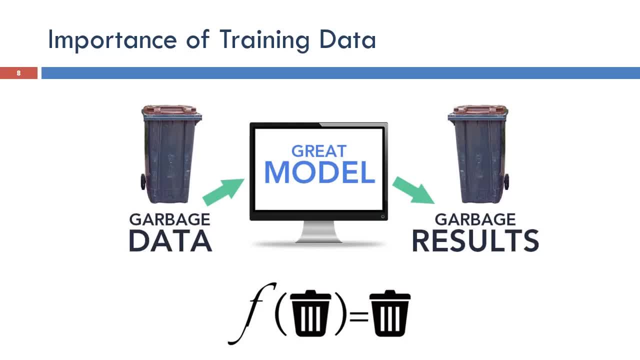 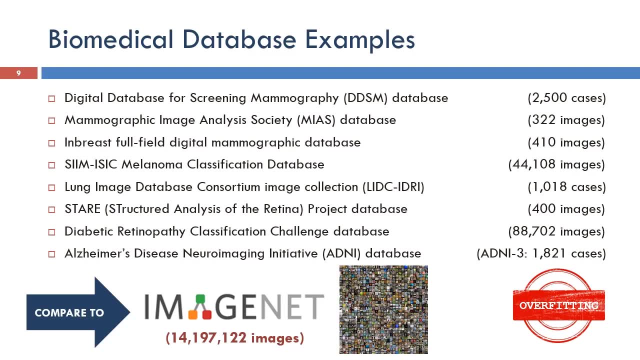 of the model can be actually uh, or the potential of the model can be realized. in biomedical engineering in particular, we start seeing now some differences between biomedical and other areas. we have so many different databases for different clinical applications. for example, we have digital database for screen mammography, ddsm database, which is very popular. 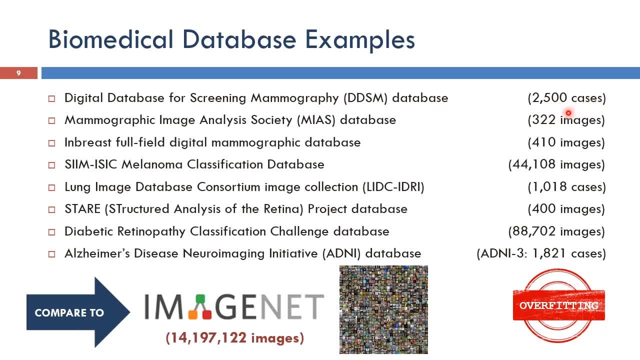 it has 2500 cases. cases means that 2500 patients or basic images from patients. you have mammographic image analysis. you have 322 images. for in-breast fulfilled digital mammographic database, it's 410. the difference between this one and the other two is that the other two here were based on film. 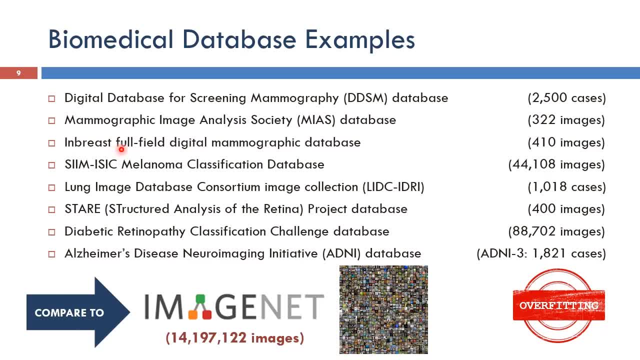 now, everything is digital. now, basically, since it's digital, it's better to actually develop the systems based on digital data. so, basically, this is: this is one of the first digital demographic databases that are currently available for research. it has 410 images only. you have other other databases for skin cancer, for example, like the isic database melanoma. 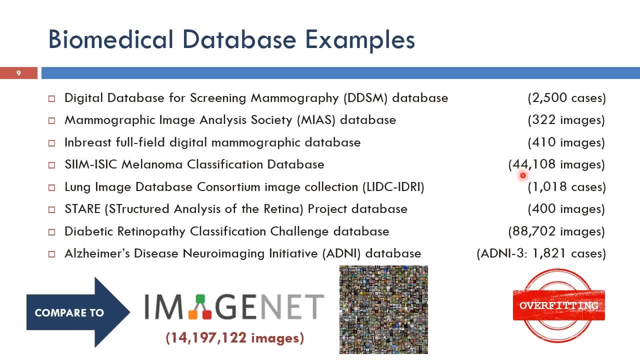 classification database. it has 44 000- a little bit more than 44 000 images. you have the long image database, consortium image collection, an idc database. it's about a little bit more than 1 000 cases. you have the stair database for analysis of the retina. it's about 400 cases. you have the diabetic. 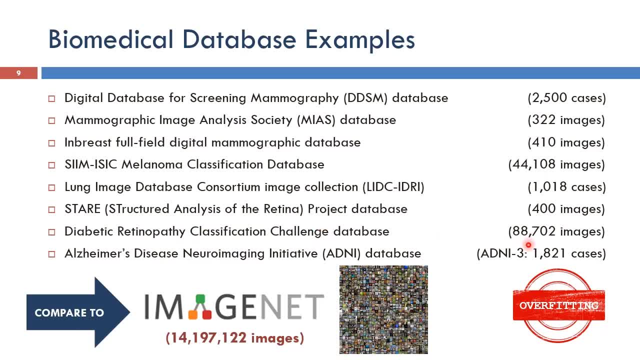 patient challenge database. you have about 88- a little bit more than 88 000 images. you have the alzheimer's disease neuroimaging initiative. basically it's about a little bit more than 1800 cases. basically, if you compare these, any any of these, actually if you compare it to whatever is, 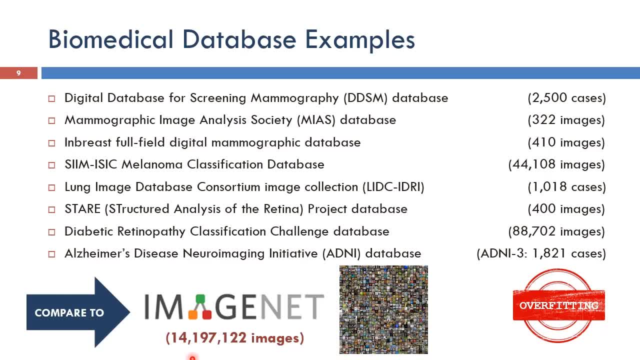 used in other applications like, for example, image net, you have more than 14 million images. if you imagine that, if you have a deep learning neural network, you have a lot of parameters. you have to have a lot of basic data points so that you can actually train these parameters. 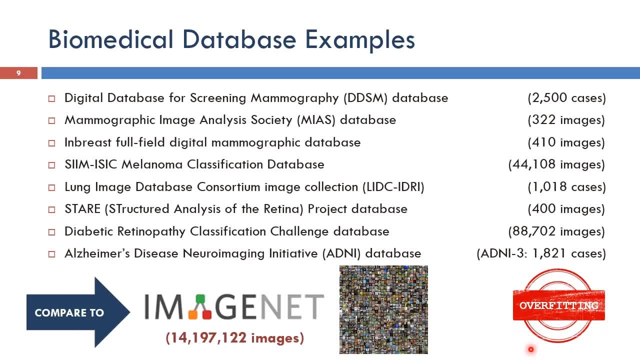 without having the problem of overfitting. overfitting meaning that you're using a model that has a much higher order than the data points that you have, and this is a potentially a very dangerous problem for the system because, basically, you can get very good results in your training. but 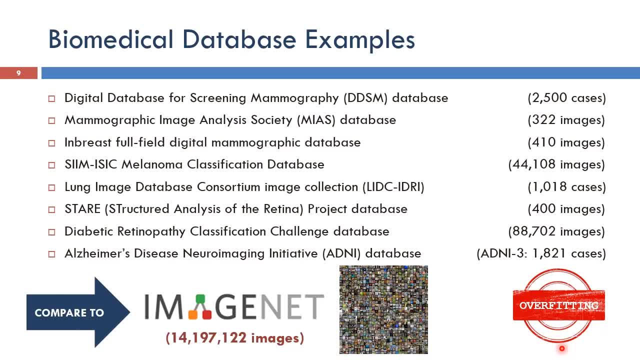 when you actually apply to real cases, you end up having very poor results. so this is one of the first concerns we have in biomedical engineering: the cases are very scarce. you don't have that many images that you don't have that many uh, for example, samples from biomedical 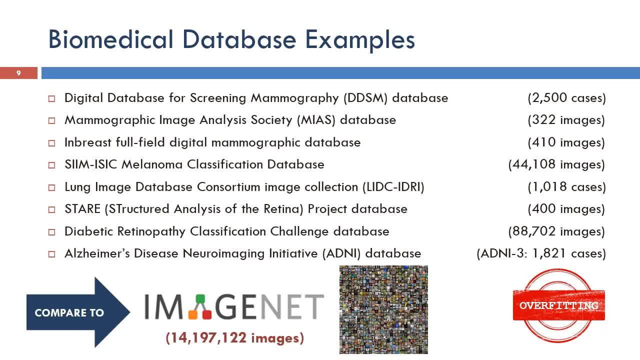 clinical data. basically because, basically, clinical data are very much protected and it's very difficult to actually collect data that is acquired in a particular way so that it can be coherent, okay, basically, it's very difficult to uh, after you collect the data, it's very difficult to actually label them in order for you to be 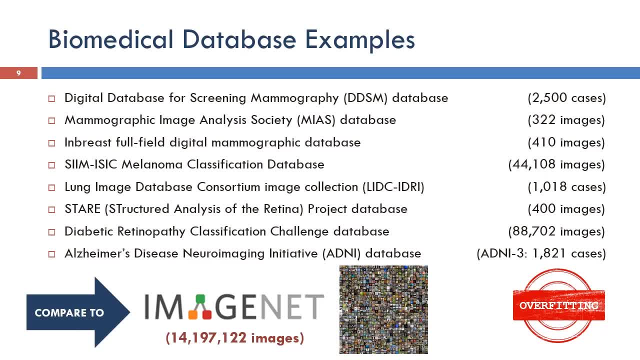 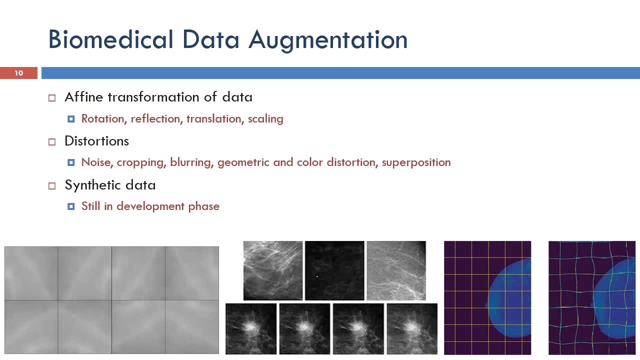 able to label them. you have to have experts and basically these experts will basically label each part of the image and basically use that to train the model. this is actually very difficult. so basically we have problems as far as the data in biomedical engineering. so, biomedical data, we try to do what's called augmentation, augmentation, we try to increase. 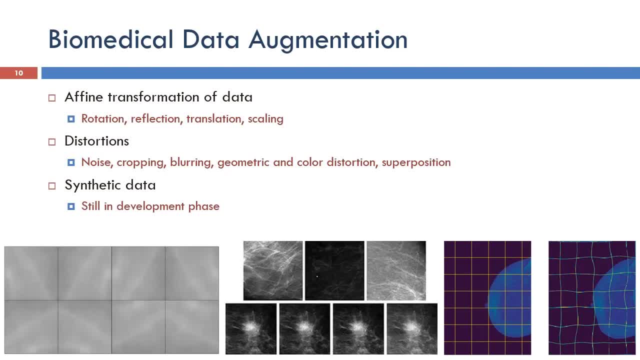 the size of our data. this can be done with, uh, or has been done using a fine transformation of data, where we actually do rotation, reflection, translation, scaling, things of that sort, just applying a fine transformation to the images, for example. okay, so if you have an image that looks like this, we basically end up. 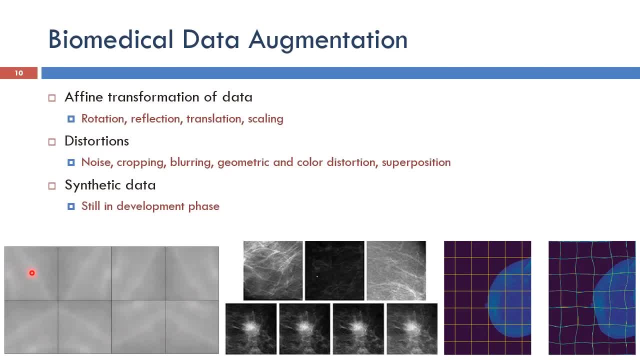 with images that look like this. basically, it's the different versions of this exact image, but actually having a fine transformation applied to them, to the deep learning system, it will consider each one of these as a different image, because each one of these points will be connected to an input node. so, basically, 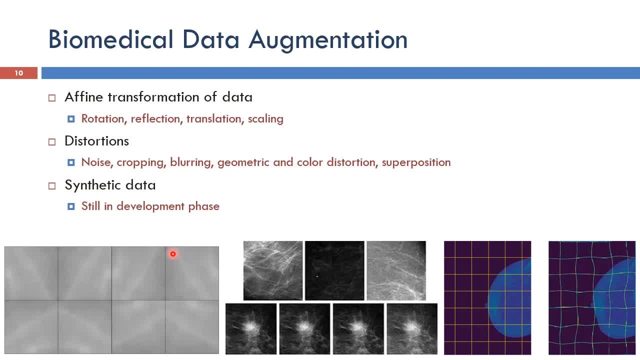 when you change the, the points which change where this point is, then the system would consider it as a different image. so basic can be very useful actually to increase the size of your data by a factor that is equal to the number of final transformations that you have sometimes actually. 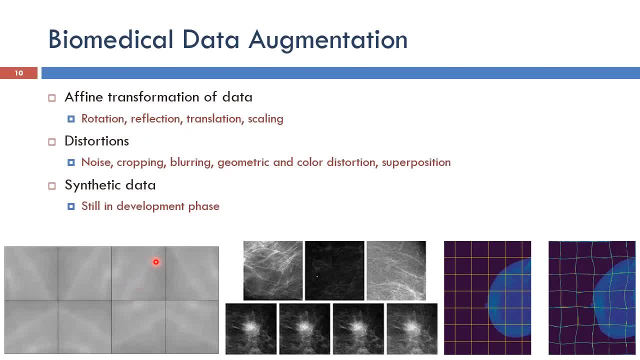 you add the translation as the translation. basically you just shift the image a little bit. okay, the scaling also can be applied, because basically if you scale the image of a tumor, it would still look as a tumor to the doctor. so basically it would actually serve as a proper sample for an abnormality, for example. 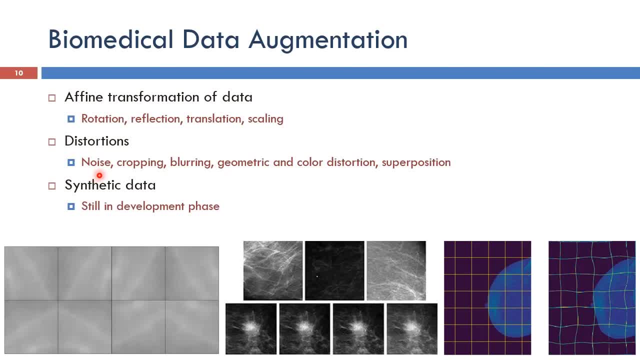 sometimes you like to also add distortions like a little bit of noise, like cropping, like blurring, like geometric and color distortion, for example. you have, uh, for example, you have the image that looks like this: you can actually uh, apply some deformation to the image so that you it looks a little bit different than the image that you have, and you can actually 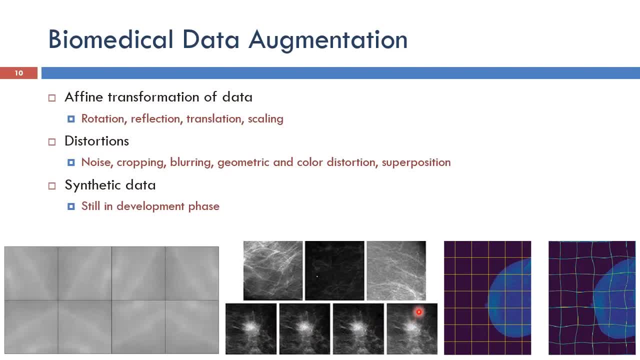 add a little bit of uh changes in the coloring of this, of the image. for example, here the dynamic region is different between these images, like here, for example. so basically, when you do distortions, you just have to make sure that whatever comes out of the distortion would actually. 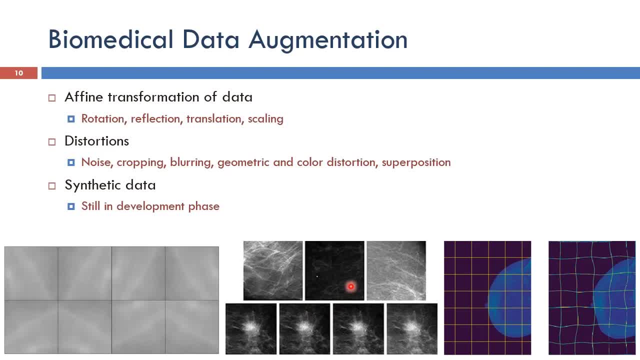 be classified by the doctor as the same original abnormality or the same original classification of the image that you applied the distortion to. so basically, you can also basically add more images if you actually apply certain distortions that are acceptable. The new thing: basically these two actually have been applied since the start of applications of 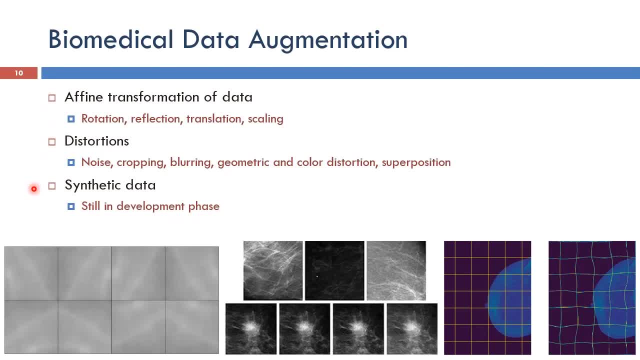 deep learning in biomedical engineering. but this last one here is still in development, where people actually try to have synthetic data. They use the original data in order to basically have a simulation program, create images that would actually be classified by the doctors as the same. 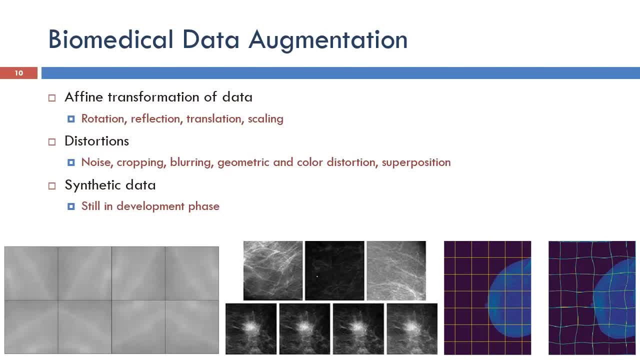 abnormality or the same classification of the original image. This is kind of debatable because sometimes you can actually add, you know, or at least make the images in such a way to make the classification look good, like basically people do that in things like adversarial example, for 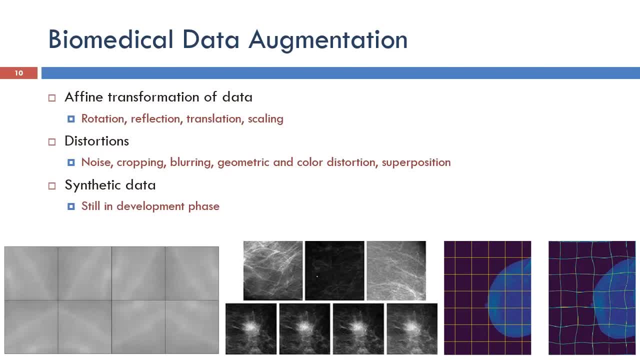 example. So basically, you have to make sure that the synthetic data is done in a way that is basically totally independent and basically totally randomized, so that we have output images that are very much usable as independent data points. Okay, this is still in development and people are not really. they are not really. 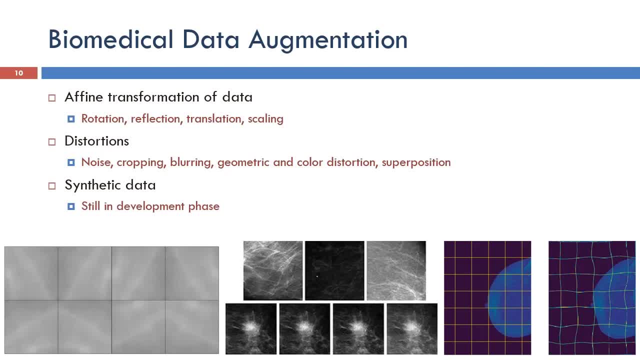 you know, approving whatever comes out of systems based on synthetic data as of now. but actually this can be a very good solution because this would open the way to having basically as many images as we want. So basically it would be a very good solution, but we have to still work. 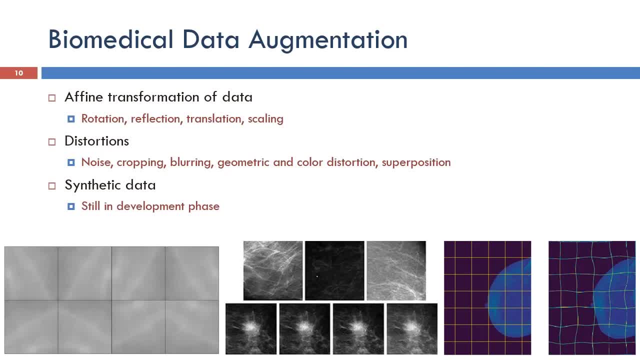 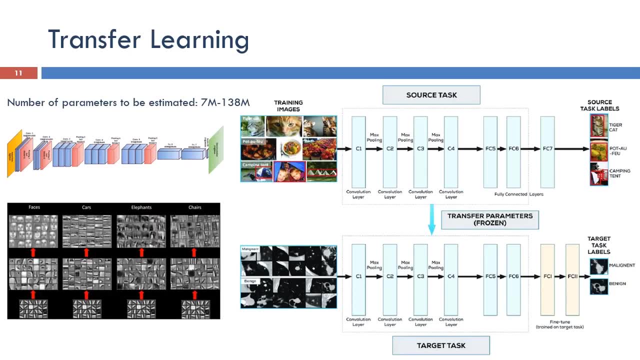 on it a little bit more in order for it to be mature enough to become useful in realistic applications. One other solution that can be used to address the lack of data is what's called transfer learning. If we have a considered realistic deep learning system, the number of parameters to be estimated is, for example, can be between: 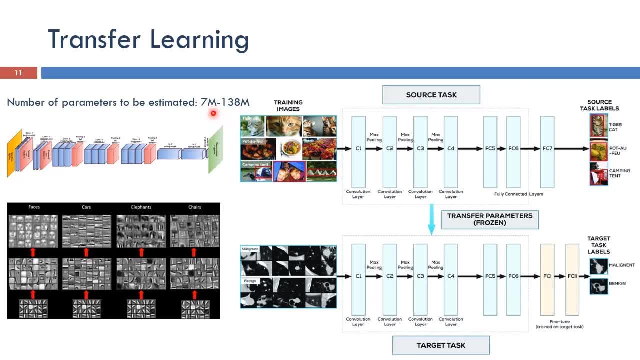 7 million and 138 million parameters. 7 million is like GoogleNet, 138 million is like VGG16,, for example, You have in the middle something called AlexNet. AlexNet is about 60, something a little bit more than 60 million parameters. So basically, you have a lot of parameters to estimate. 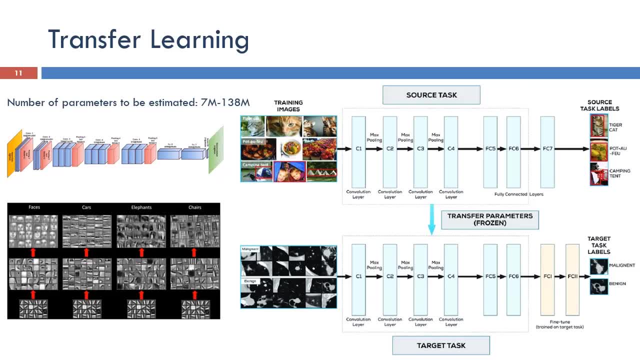 If you're trying to estimate all these parameters using, for example, a 300 images or 322 images, like the miniMIS or MIS database, this is kind of difficult and definitely overfitting would be a major problem in this case. 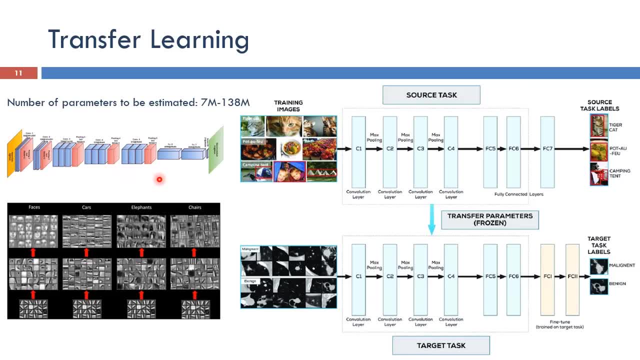 So people had an observation that you have basically for the deep neural networks. you have- actually most people use something called convolutional neural networks at the beginning and then you have fully connected layer at the end. okay, for connected layers at the end. 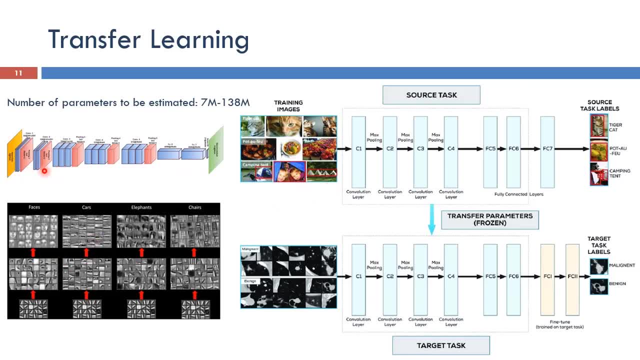 So, basically, if you look at the output from the convolutional layers at the beginning, you will find that they are very much independent of the kind of data you use. For example, people train the same network with faces, with cars, with elephants, with chairs, and basically you know as you go deeper. 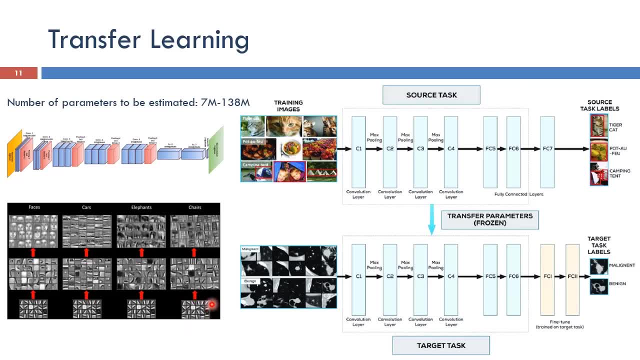 you basically find that the deeper layer would actually end up looking like, for example, very similar. These look very similar between the different different applications, basically. okay. So basically you have different basic features that are present in all images, like edges, for example. okay, and use these to basically train. 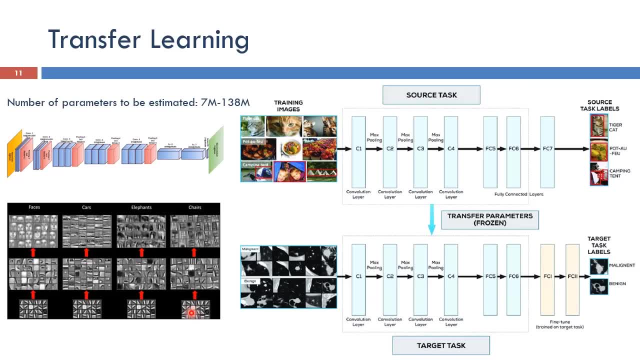 the network to classify these objects, you know, whatever they are. So the idea here was we can basically get the first layers, you know, the layers that are not relevant to the particular data we use, and basically transfer them, as is. So, basically, we can use a GoogleNet, for example, or AlexNet. 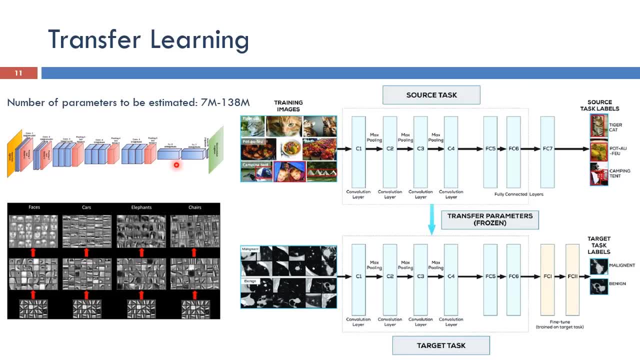 that is trained on the huge ImageNet database that has 14 million images, and basically just transfer the first few layers as is And then in the final layers that classify the particular object that we have. for example, here we have different, like tiger, like cat, whatever, okay. 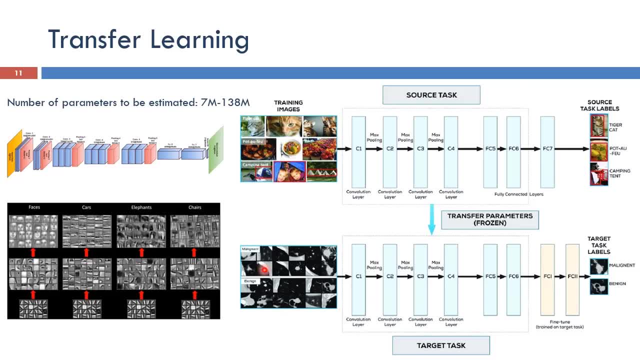 we can actually train the final layers only with our own particular data, so that we can basically, instead of having like a hundred or a thousand classes, like in ImageNet, for example, you have only Malignant and Benign, And when you do that you have a very good network. that actually with the parameters here. 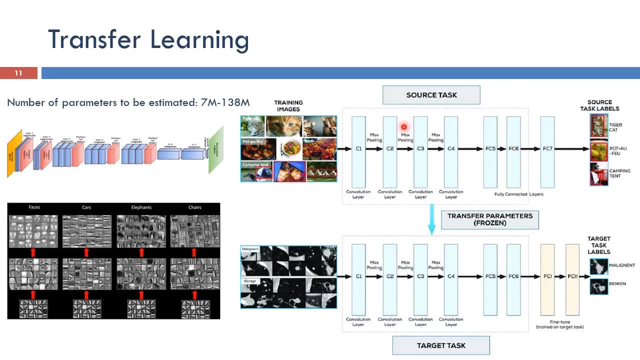 most of the parameters were actually trained by a very large database and basically only adapted or customized to the particular application we have in biomedical engineering, in the you know the last few layers, Like, for example, the fully connected layers and the classification at the end where you have the classes basically. So basically, 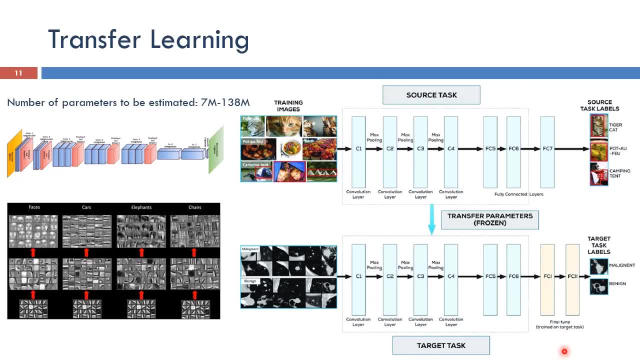 this can be a very good solution whenever you don't have enough data to train the whole network with your data. If you have enough data, definitely go for it, Go for training the whole thing, But actually if you don't have enough data, then you just have to do transfer learning so that you can. 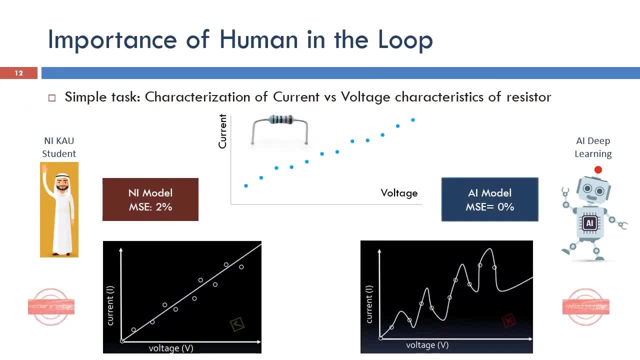 minimize the problem of overfitting. Many researchers actually observed that in many AI systems it's not enough to just have the AI system working by itself. There is an importance for having a human being- or you know what's called human- in the loop, where the human actually observes the. 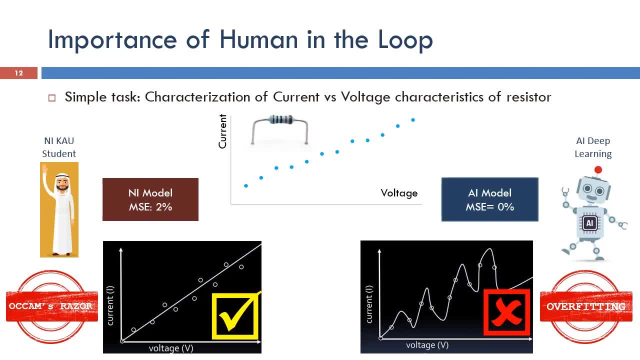 operation of the neural network And basically adjust for any obvious deviations that might come up from the training of the data or from the output of the system, for example. Let me give you a very clear example to see how important this is in a very basic task, And you can imagine that this example would actually carry. 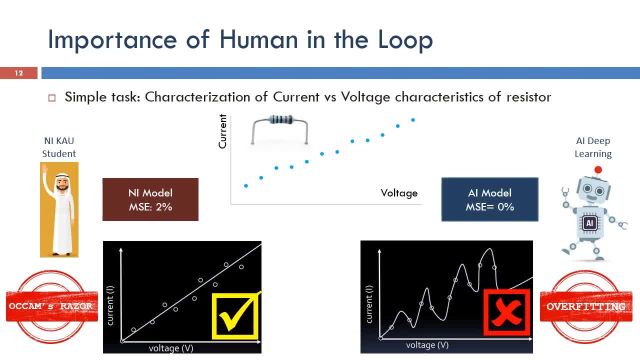 on to the diagnostic. you know problem in biomedical engineering: If you have a student and an AI system, ask to. basically, you know, ask them to do a very basic task And you can imagine that basically you give them the data from a resistance. We have the current and the voltage. 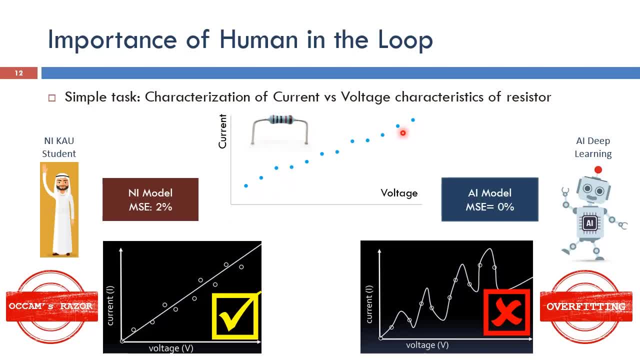 waveform from resistance. You have as many points as you want here, Okay, And basically you ask the student and the deep learning system to basically come up with the model that would actually describe this data. This data basically Okay For the AI. it would try to minimize the mean. 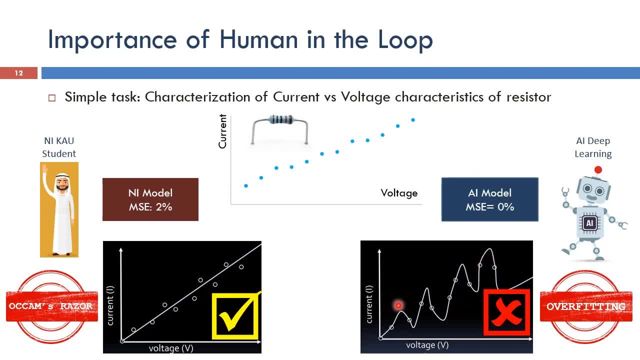 square error. So basically, it comes out like this: because actually you have so many different parameters, You can actually, you know, have a curve with an infinite or a very large order, And you can basically make all the points actually, or make the curve that comes out of the model that you. 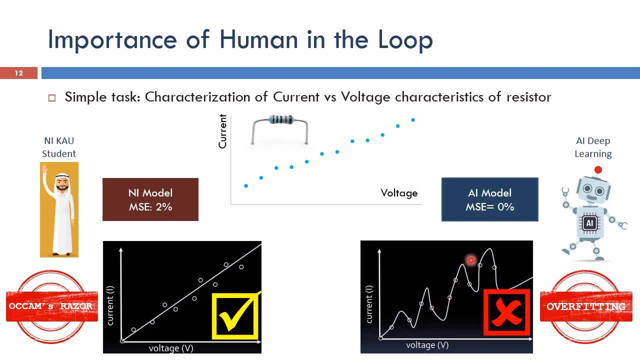 develop from the AI system. pass through all the points And basically this is a big problem because this is not really what we should have in reality, What we have in reality. if you have a smart student, like our students, basically you would realize that this is a 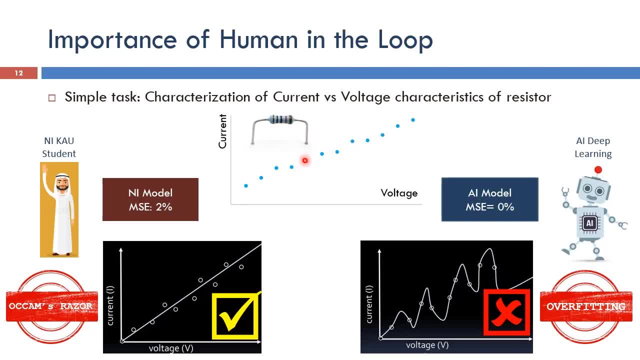 resistance. So the model should follow what's called Ohm's laws. It should look like a linear system. So basically the student would right away develop the or estimate the linear, the straight line that passes through the points, and minimize it at mean square error. Okay, So basically this is: 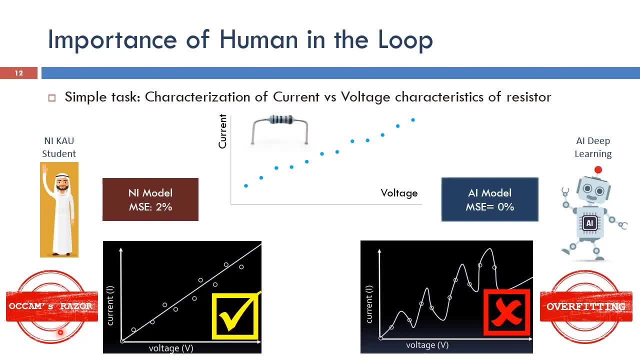 what's called Occam's razor. Occam's razor basically talks about that the simplest solution or the simplest model is usually the right one and generalizes better. So basically, this model actually would generalize better. So, basically, this model actually would generalize better. So. 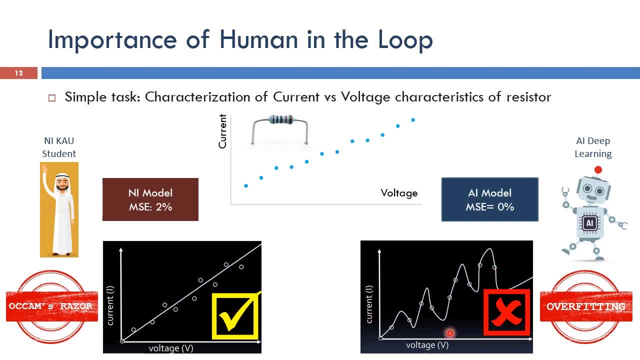 could represent this kind of function in a lot of different ways, And this method is忍n d actually delineate these two ways as described in the hundreds samples. So basically, you generate and you output rehearsal, which is very important. So everything you do here and exactly that much better than this one here. Okay, so this one here is good, This one here is bad, And basically, without a human observing the performance of the AI system, you would end up having things of that sort, But unfortunately, for very large neural networks, it's very difficult to observe them. okay, here, because the Day times only two dimensions have one dimensional data, basically actual. you have a variable, dependent variable and then independent variable, and that's it for GPU networks. you have hunted, Collecting ages ten years. you have in so decades, sixünge. 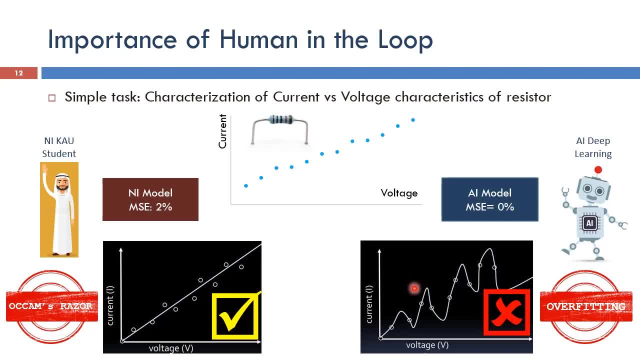 is very difficult to observe them. Okay, so basically here, because the data is only two dimensions, have one dimensional data, basically actual. you have a variable dependent variable and then independent variable, and that's it for GPU networks. you have collected thousands of input variables and you have, as we saw, millions of parameters. so 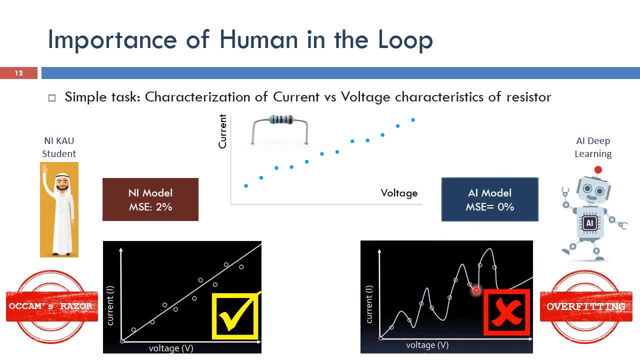 it's extremely difficult to observe if things like that happen, but we can observe things of that like that when they happen because of the overfitting that we see in the results. so basically, if we give the model another point, for example, or basically tested the model with independent data, the data that the 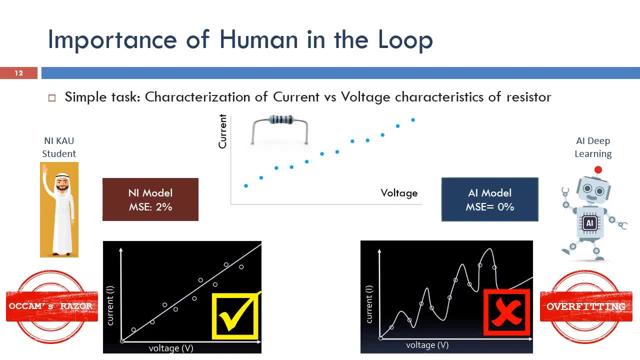 model didn't see before would realize it very, very clearly that we have a problem in our model. so basically, we have to have a man in the loop or a human in the loop in order for us to be able to regularize the operation of the neural network. okay, for diagnostic, basic diagnostic cases, for example, it's not. 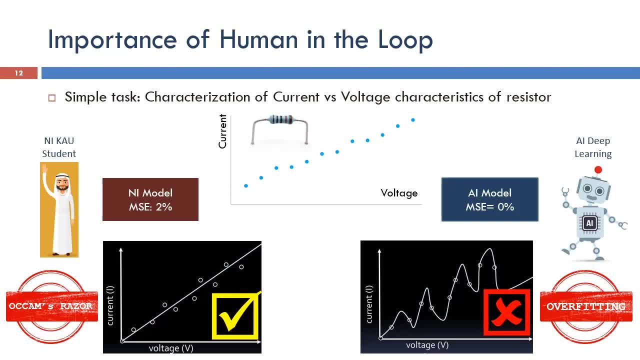 enough for the, the AI system, to just basically give a diagnosis and we accept it. it doesn't work that way. we have to have a human in the loop, and we have to have a human in the loop and we have to have a human doctor that would look at the data and look at the output from the AI. 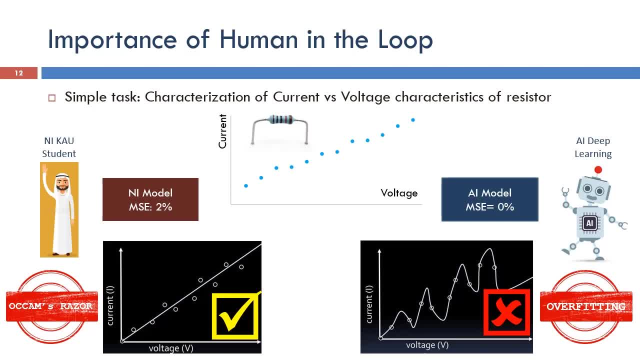 and then confirm the output of the AI or dismiss it, okay, based on the clear or obvious problems that he sees in the data. so, basically, this is very important. having a human in the loop with AI systems is very much a clear you know mandate and biomedical engineering applications. 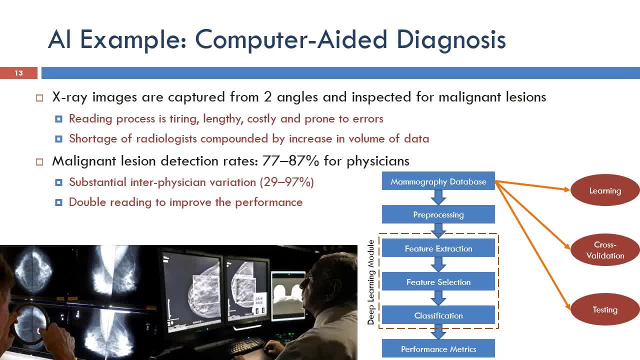 now we're going to consider a very particular AI example from biomedical gene, which is computer aided diagnosis, in order for us to understand a little better how AI systems are utilized and how they can fall into problems. you know, without even basically technically we don't see how. 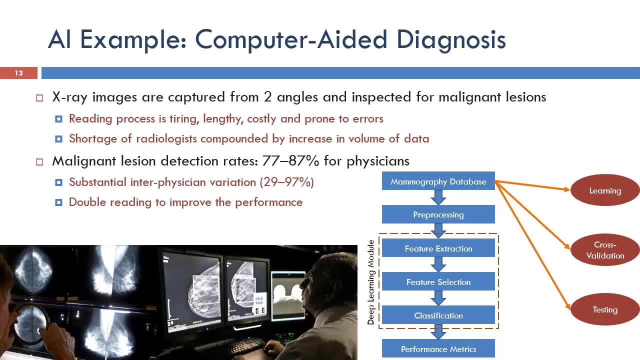 it can happen, but actually in reality such problems can happen. so if you consider, for example, computer aided diagnosis of mammography: basically acquire two x-ray images that are acquired from the computer and then we can, we can, then we can see that the patient is actually operating on two different angles, usually cranio-codal. 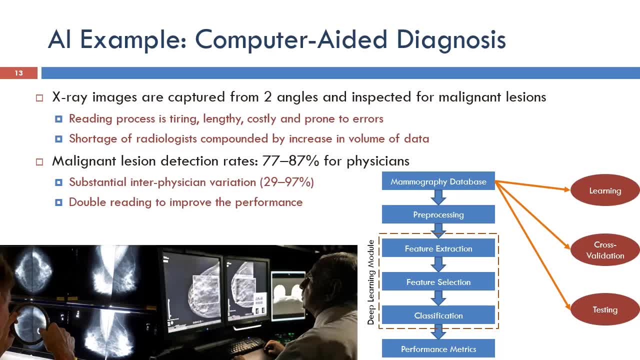 and medullator oblique images and they are inspected for malignant lesions. usually the reading process is very tiring, it's very lengthy, it's very costly because doctors are paid, you know the hourly rate of doctors is really high and definitely prone to errors because basically not because of the doctor expertise, which is actually a factor, but actually because of the level of the patient's condition is really high and 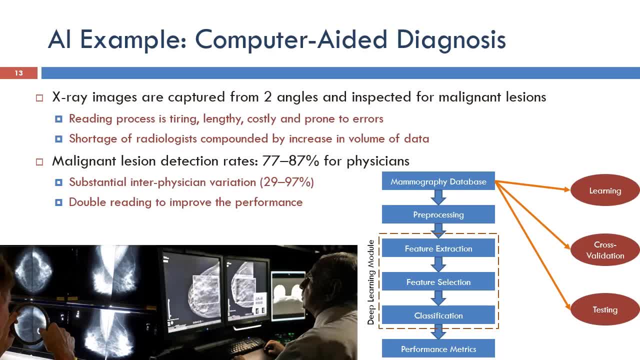 basically, if you have the image presented to the doctor at the beginning of the day is different from presenting the same images after eight hours of reading. basically okay, The doctors get tired and basically their performance changes with time. So another problem that would actually. 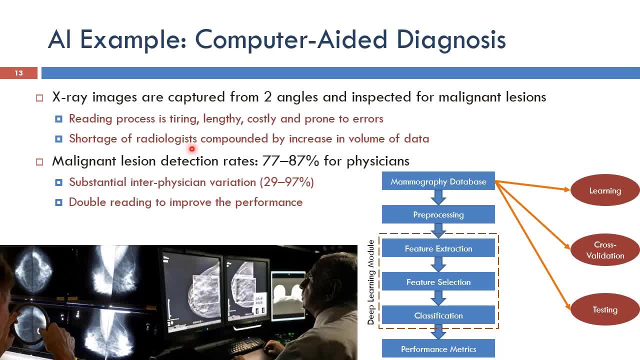 complicate this is that we have a shortage of radiologists- okay, The radiologists actually are among the specialties with very few doctors, okay. And basically the shortage of radiologists actually is even compounded more by the increase in the volume of data. Now, imaging systems are. 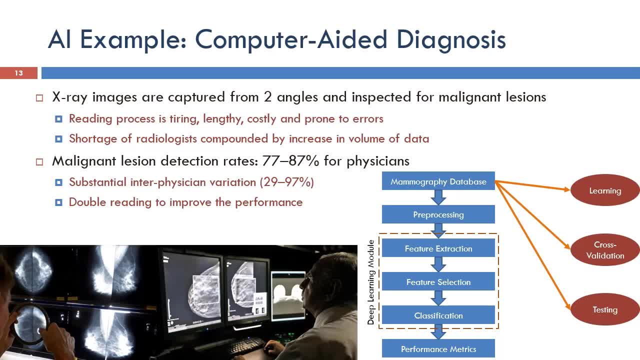 everywhere We have, instead of 2D images we have 3D volumes. So basically we have many more images for the doctor to read every day, and we still have. we don't really have enough radiologists available to do that, So basically it would make. 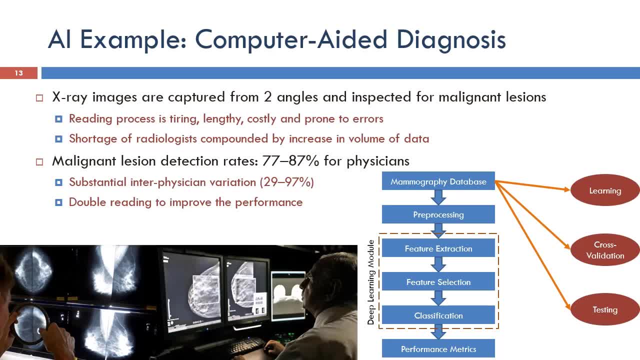 sense to have a system that would assist, not replace, assist the doctor, okay, Which is really important. okay, Just to be able to also, you know, motivate our, you know our- development of computer-aided diagnostic systems. malignant lesion detection rates are between 77 and 87 percent. 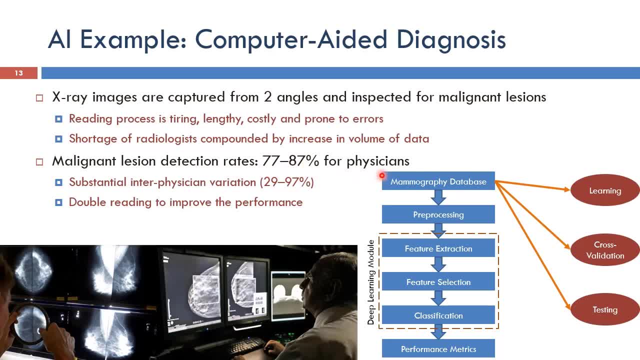 depending on a lot of things, including the physicians, okay. So basically, among physicians, the average rate is basically maybe 80 percent. okay, The problem is that we have a substantial inter-physician variation. So basically, if you look at doctors, if you look at individual doctors, the rate might be between 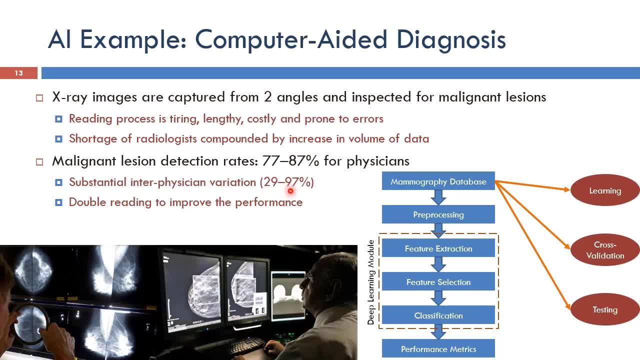 29 percent and 97 percent, depending on the experience, which is really a very wide variation, And so people use double reading to improve the performance. It's not enough for one doctor to read the image. usually two doctors might read one image and it's a lot of work, But it's not enough for one. 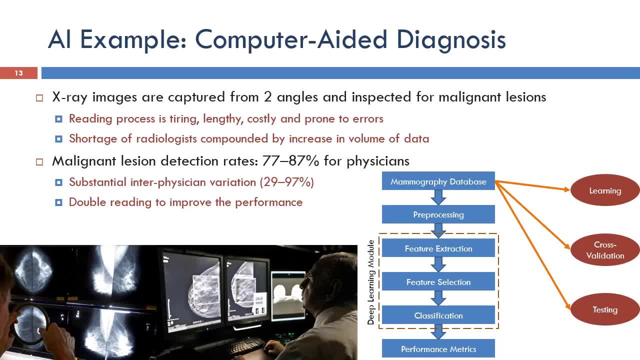 doctor to read the image. usually two doctors might read one image and it's a lot of work, But it's a lot of work, But it's a lot of work, But it's a lot of work. If two doctors- you know, if you can have two doctors- read the image, it would actually improve the performance because it might basically allow one of the doctors to at least catch the problem in the images. okay, 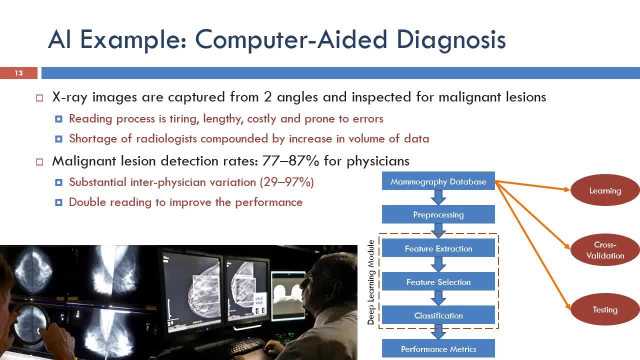 So basically, this is very important. So basically, this is another factor because we are now doubling the effective volume of the images, because each image has to be read by two doctors, not just one. okay, So basically from this we can see that computer-aided diagnostic systems can be very useful as a second reader, for example. okay, 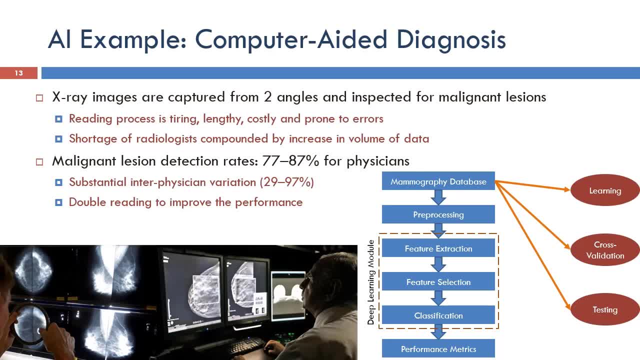 So basically you can read the images and the physician reads the images and then we compare the two. The doctor actually looks at the report from the CAD system and basically if he misses something or he actually observes something that wasn't there in the computer-aided diagnostic system output, it would still be caught and basically the diagnosis would come out right. 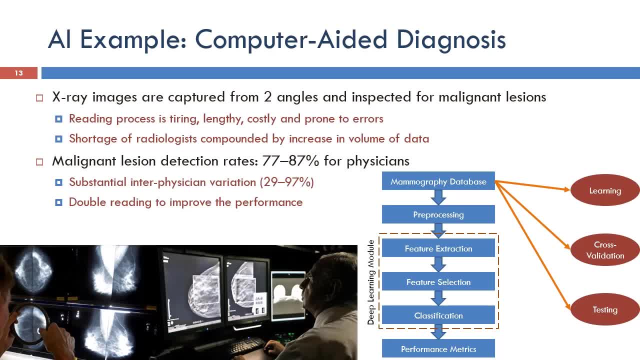 In order for us to build a CAD system for such application as mammography, we have to have a database, and this database, as we saw, we don't have so many images, but we have to actually divide what we have into three different categories. 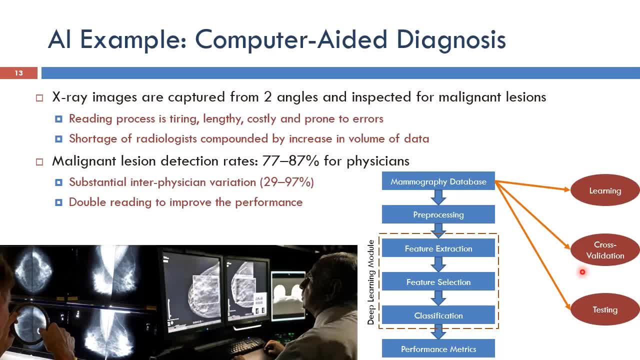 We have to have a learning set and we have to have a cross-validation set and a testing set. The learning set would be used to teach the system how to work. The cross-validation would actually help optimize The parameters of the system while it is in training. 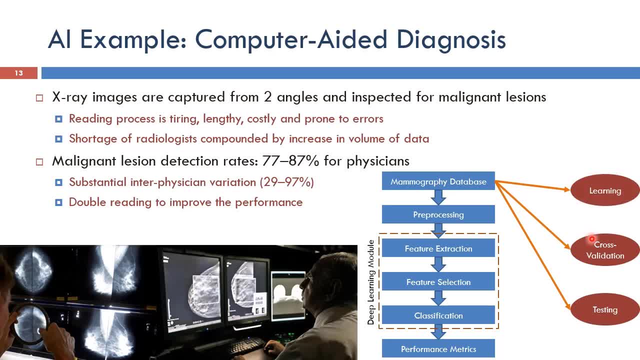 So basically, I basically use the learning data and then test it on the cross-validation. If it doesn't work properly, then I adjust the parameters and work again and basically keep working in this cycle until I get useful results or good results. Then, in order for the system to be tested properly, we have to use independent testing data, data that the system never saw. 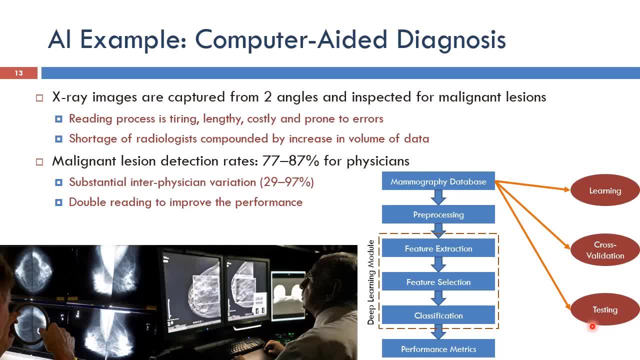 So basically, we use testing data to catch such things as overfitting. Okay, so the results from the testing data would be the actual results that would be expected from the system. We usually take these images and pre-process them. There are a lot of things that can be done, including density correction, including if you have some kind of noise, for example, you can actually do some denoising. 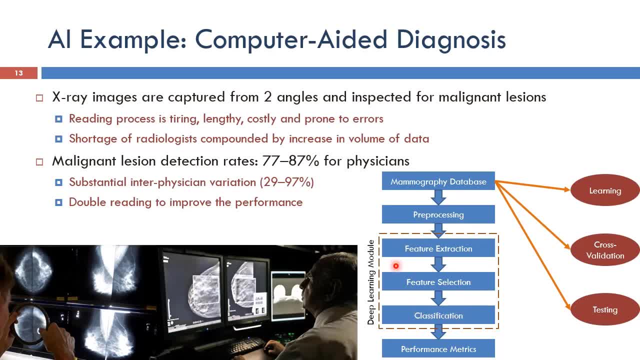 And then you enter that into The machine learning system, which can be basically a statistical learning system or a deep learning module. If it's a statistical learning system, then you have to extract features, You have to select which features are useful and then you have to design classifiers to basically use these features to classify the different classes in your data. 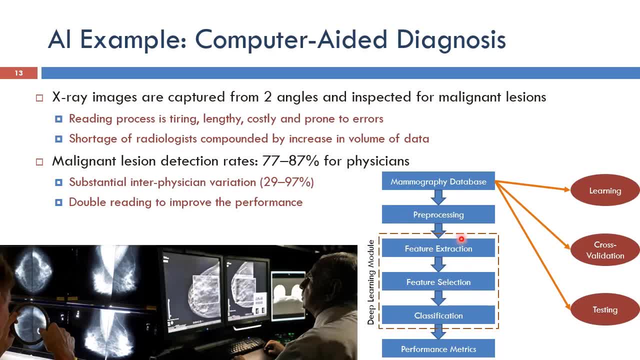 If it's a deep learning module, then basically all these are included in the black box where we actually enter the data and basically get the output Right. So we don't really design these things on our own. They are basically learned from the data. 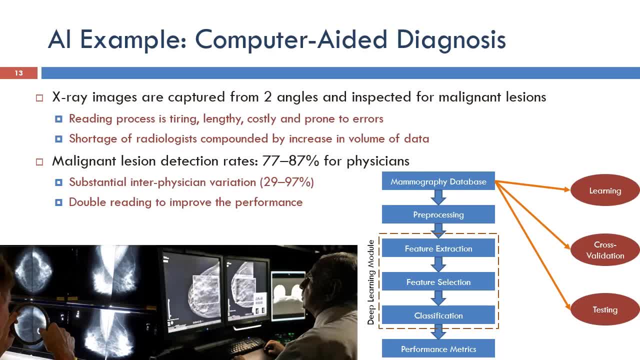 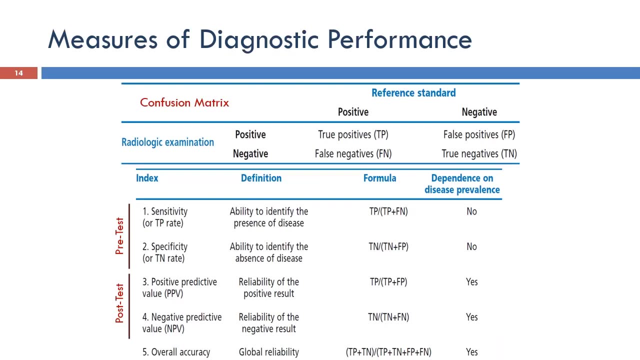 After that we have to have what's called performance metrics. People think about the accuracy as the performance metrics, the performance metrics, But actually, as we were going to see, this is not enough. In biomedical engineering, it's very difficult to have a misclassification. 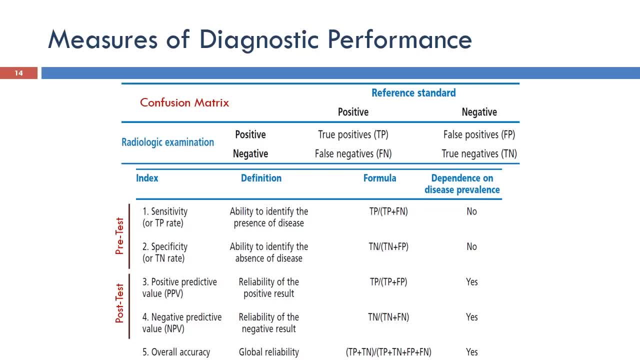 If the case was positive and you classify it as negative, then for mammography for example, the woman would go and get a clean bill of health and sent home and then comes back in a year or so with a much worse case and might not be able to basically do much at this point. at this later point. 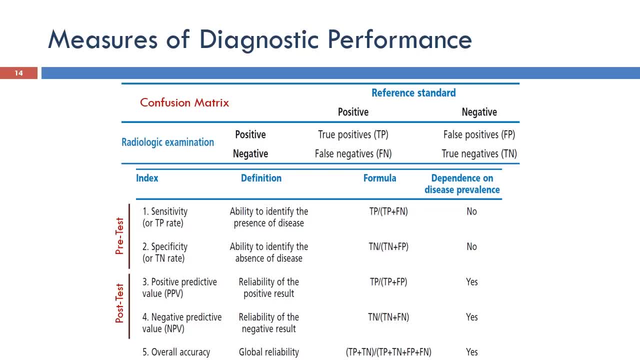 So basically, we have to have differences between basic. We have definitely have true positive, We have true negatives. This is what's called The confusion matrix, And we have false positives and we have false negatives. OK, for the false positives, it means that the woman would be basically told that she has a problem and she might have to end up doing a lot of further investigation that might be invasive. 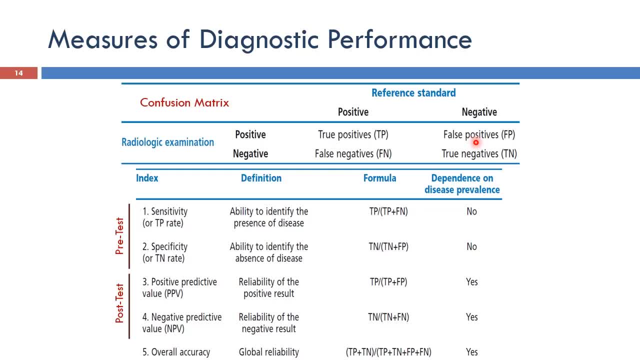 But at the end she would be told that nothing is wrong. So basically everything is OK here. for the false negatives, This is a bigger problem, where you actually tell the woman that She's OK and she goes home and basically stays for a more, more time, like a year or so, and comes back with a deteriorated case that might not be basically treated at this time. 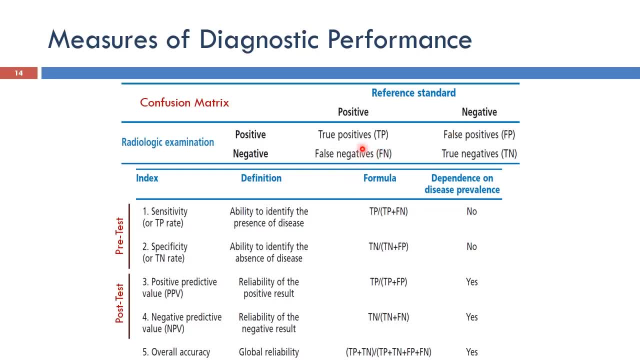 So, basically, this is a big problem. So, in order for us to be able to not just add these over the whole thing, just to get the accuracy, we need to actually discriminate the false negatives and the false positives. We can do that with the so-called sensitivity. 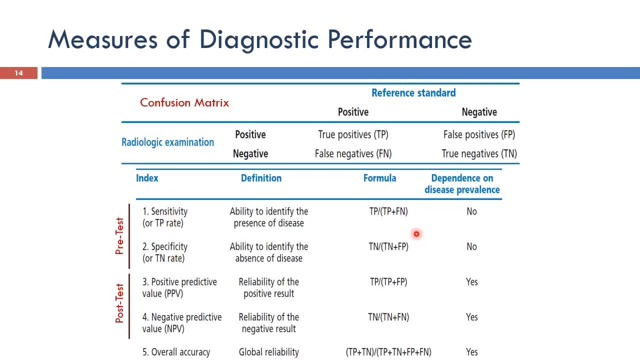 And specificity. sensitivity or the true positive rate is basically the true positive over the true positive, plus false, negative, OK, so basically this is a reference standard. This is the true OK cases. all these cases are actually supposed to be positive. 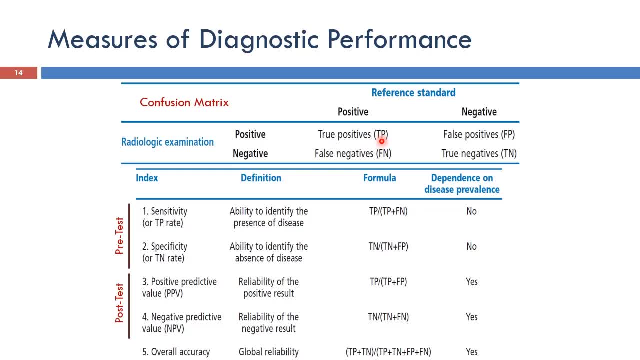 So basically we have to have all of these as TP. So when I divide TP plus over TP plus FM, I basically got the percentage of the actual Uh women with cancer that I was able to say that you have cancer. OK, this is very important. 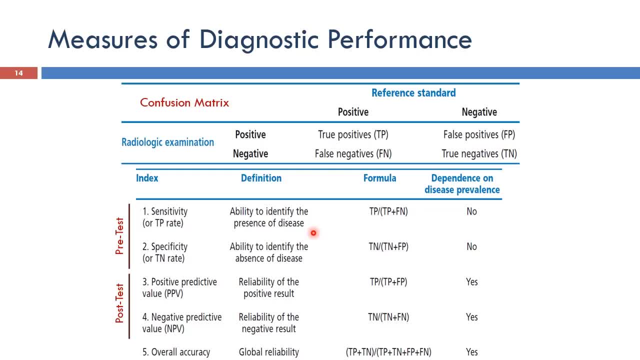 The specificity, on the other hand, looks at the negatives. Basically it's the ability to identify the absence of the disease. So basically here it's TN over TN plus FP. So basically the specificity means that when it's high, then basically I can identify the normal cases from the. 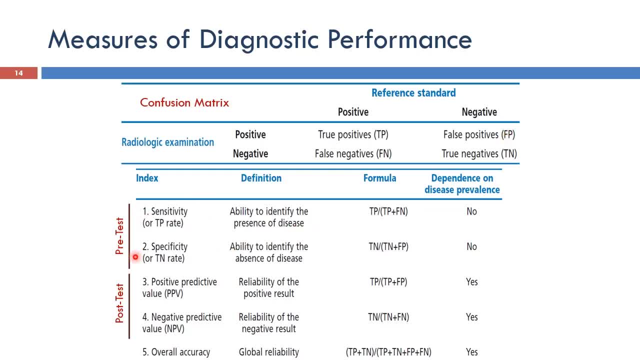 Uh, Uh, Uh, Uh, Uh Uh, false positives. basically, These two are called the pre-test matrix or pre-test parameters and basically whenever a woman is going to do an investigative radiology, for example, it chooses the particular test that provides the high sensitivity and high specificity. 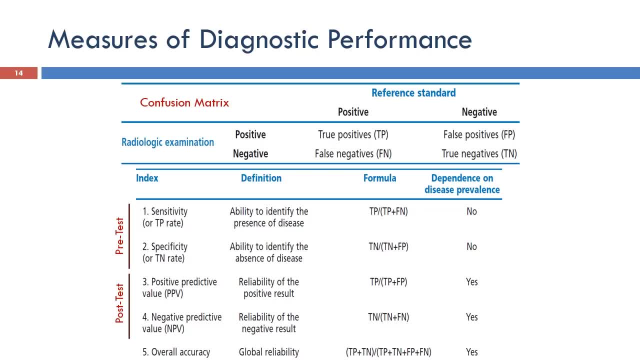 OK, so basically this is very important. OK, After the woman does the radiology and basically the results comes out, the results from this particular technique comes out. we have what's called post-test parameters or post-test metrics or measures. okay, 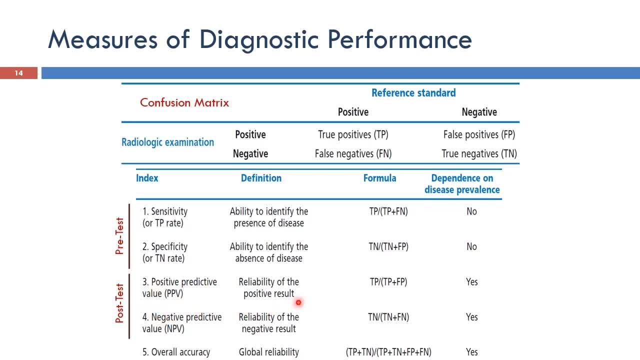 We have the positive predictive value and the negative predictive value. This talks about the reliability of the positive results, meaning that if I get a positive result, what is the percentage, what is the likelihood that this positive result is actually positive? okay, If we have a system that would give. basically, 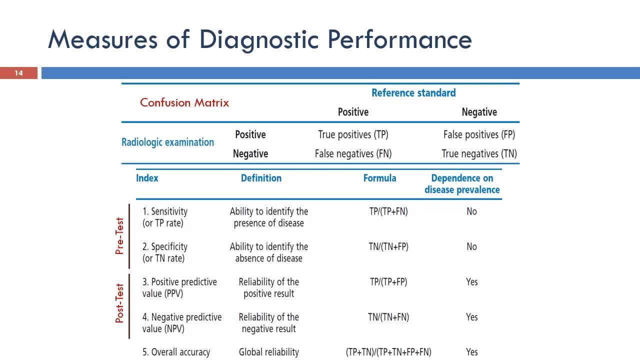 all the cases as positive. for example, then a lot of cases might come out positive but they are actually negative. So basically, this would give you the reliability of the results, of the positive result in particular For the negative predictive value. 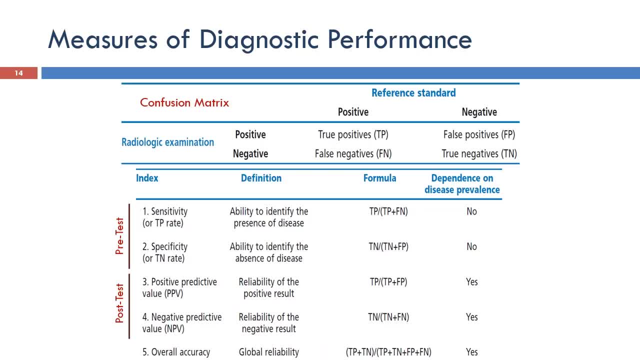 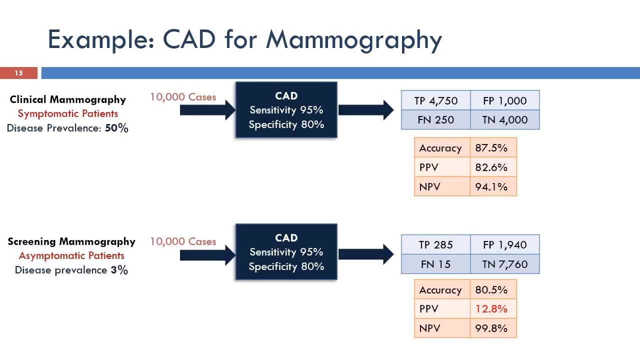 you talk about the negative results, And this is very important. This is, give a very specific numerical example so that we can actually realize the importance of these kinds of measures. If we have a CAD system, if we design a CAD system and basically this CAD system had a sensitivity of 95%. 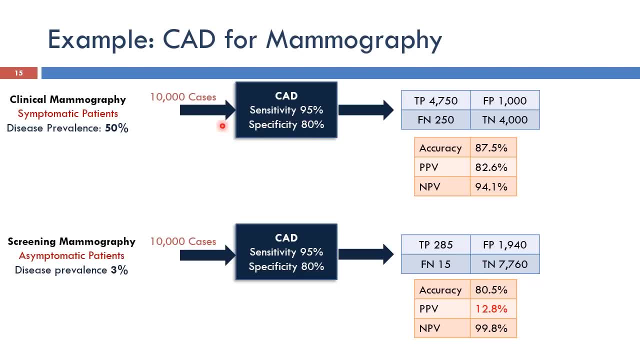 and specificity of 80%, meaning that if we have, for example, 100 cases with cancer, it would detect 95 of them. If you have 100 cases that are normal, it would say to 80 of them that they are normal. okay, 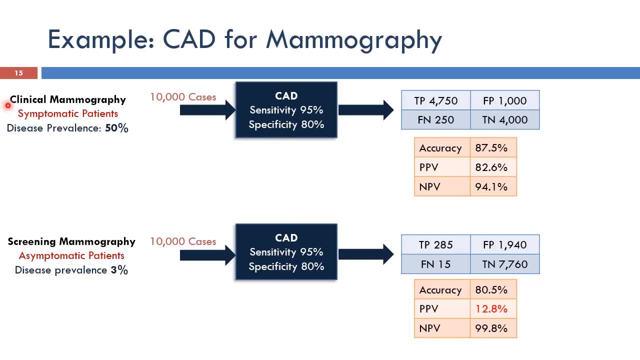 And basically we use this system twice And we use it in situations called clinical mammography once and a screening mammography once. Clinical mammography where you have symptomatic patient, a patient that comes with a complaint, for example a mass. 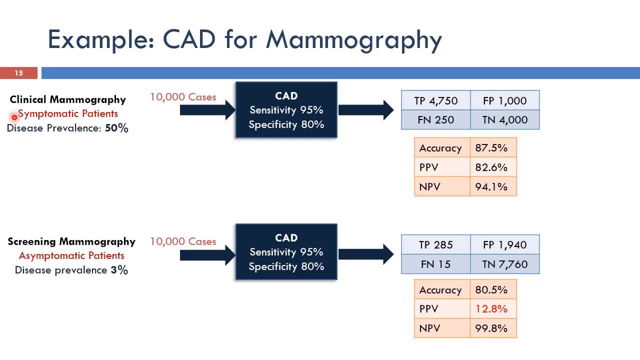 She has a mass, okay, So we would like to use clinical mammography in order for us to identify whether this mass is benign or malignant. okay, So in this case, for symptomatic patients, there is a very important parameter called disease prevalence. 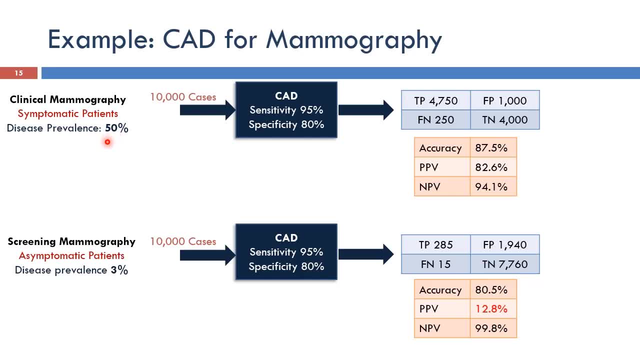 And the percentage of symptomatic patients that might have a problem or might have cancer is 50%. okay, Because they have a lump And this lump is like 50-50, basically, 50% normal, 50% abnormal. On the other hand, if you have asymptomatic patients, 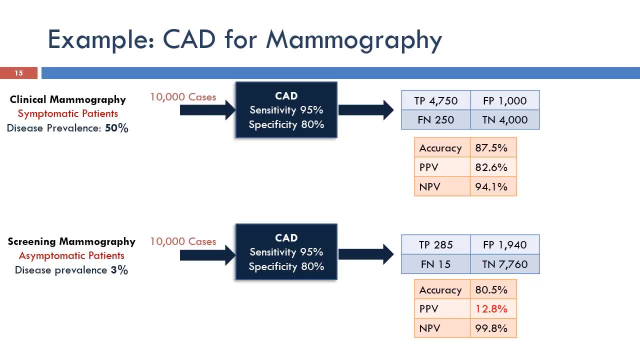 for screening mammography, like the screening programs that people actually adapt these days, where women go every year or every couple of years to do mammography just to make sure that no initial signs of cancer, no cancer, appear in the mammograms. And if they appear, you can actually catch them later. 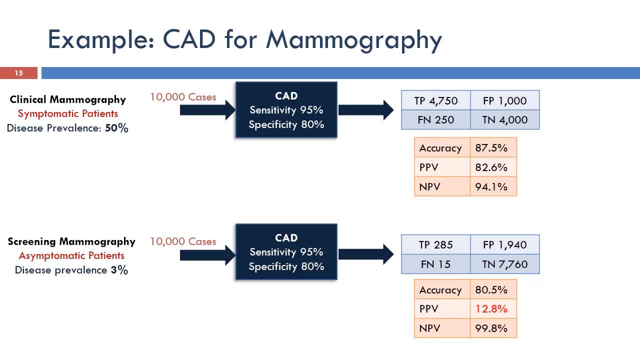 early on and basically treat them before they become a problem. So the disease prevalence in this case is only 3%. If you do the numbers, if you basically crunch the numbers here, you develop the confusion matrix first and then compute the positive predictive value. 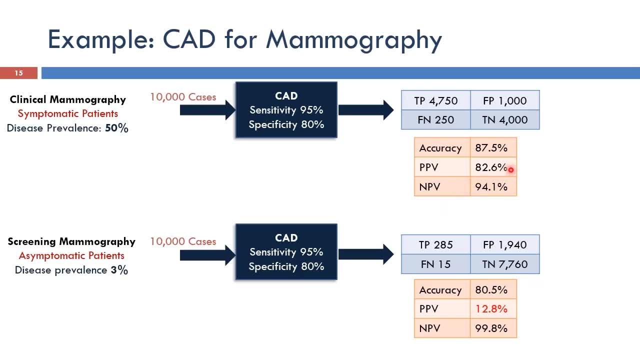 and negative predictive value here. you see that here the positive predictive value is about 82.6%. The negative predictive value is 94.1%. The meaning of this, the positive predictive value here, is basically very much different from here We have: the positive predictive value here is 12.8%. 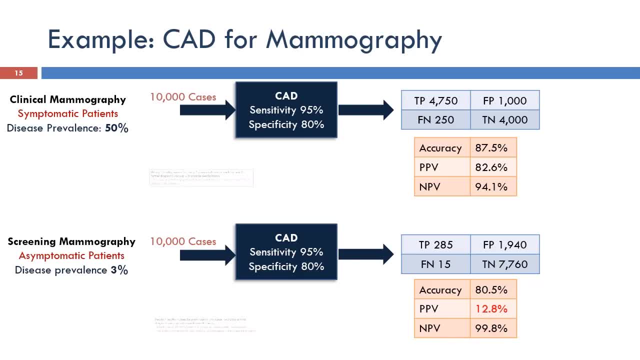 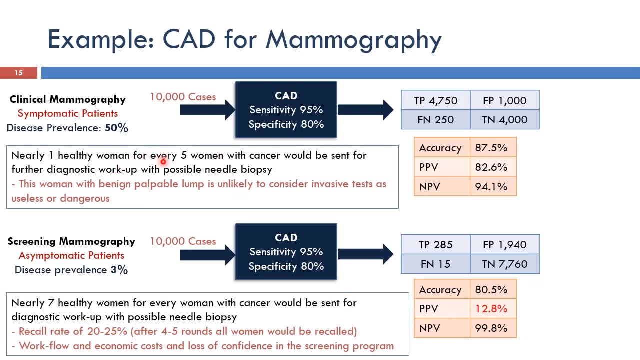 and negative predictive value here is still high, over 90%- 99.8%. The meaning for this is that, based on these results, for every healthy woman with cancer, for every healthy woman, for every five women with cancer, you have one wealthy woman. 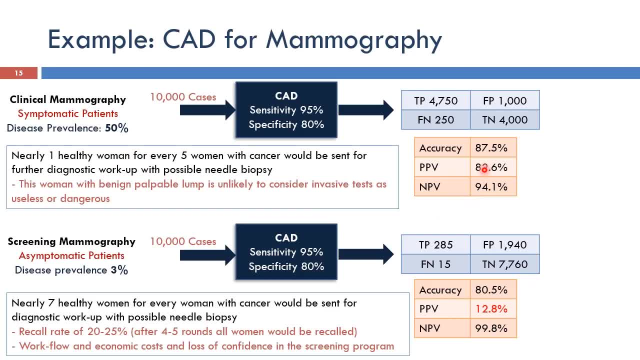 because you actually have the percentage, almost 80%, meaning that there is an error of 20%. It means that if you say that this woman has cancer, basically one out of five, basically, would be actually diagnosed with cancer, but she doesn't have cancer. 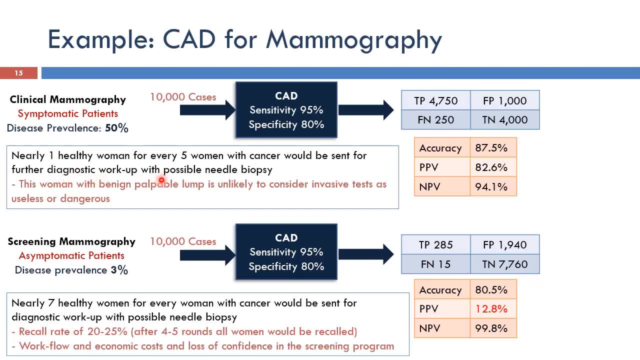 This woman actually will have to endure diagnostic workup and possible needle biopsy, which is kind of an invasive procedure. Just get a sample from the location of the lump just to make sure that it's benign or malignant. It's sent to the lab and basically analyzed. 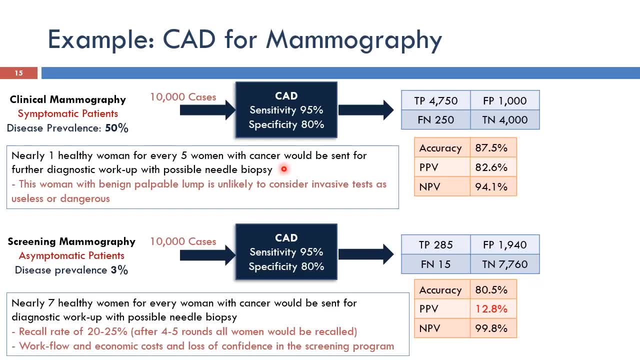 for cancer science And in this particular case, since this woman has a lump and want to make sure that this lump is benign, she would not mind that because basically, the results that come out from the lab testing is basically the gold standard. It's 100% accurate. 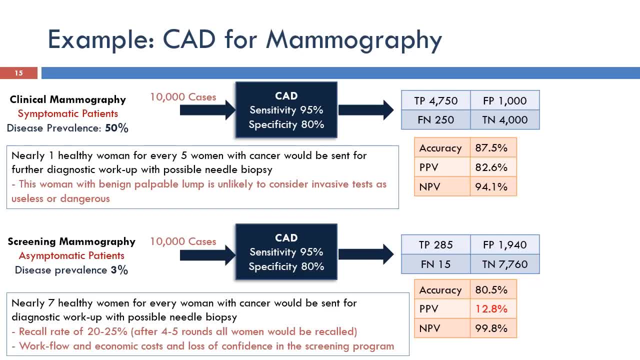 If it's okay. if it's benign or malignant, then it's final decision. now It doesn't have to actually worry about this anymore. So basically, in this case it can be acceptable for the woman, okay, And doesn't consider the additional workup. 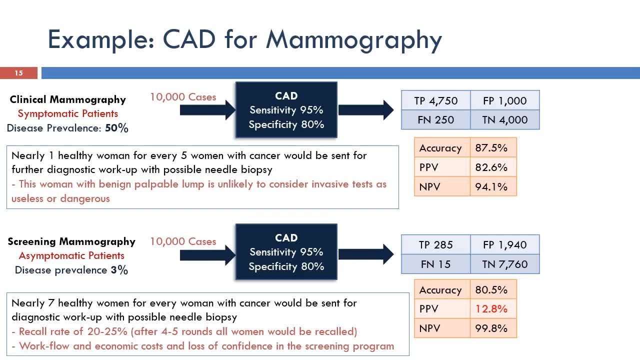 that she will have to endure, or the needle biopsy as useless. Basically, you consider them actually as necessary to make sure that she's fine, that she will be diagnosed with the right diagnosis. On the other hand, here you have the positive predictive value of 12.8%. 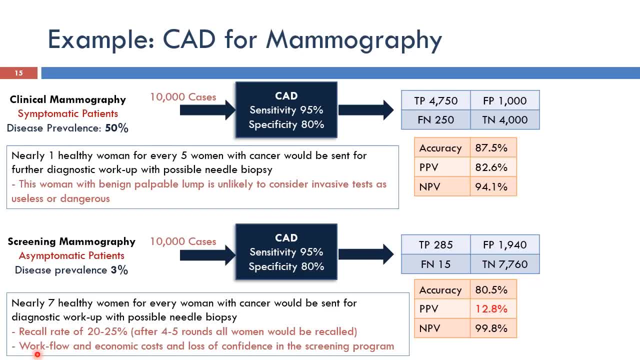 meaning that for every woman that has cancer, seven healthy women are basically diagnosed with cancer incorrectly. This is a big problem, meaning that basically each time you're going to have a round of screening mammography- about 20 to 25%. basically the false positives here about. 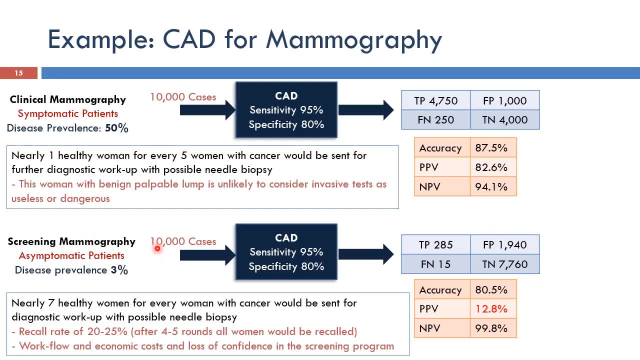 see here it's about 20 to 25%, Very close to 2,000 out of the 10,000 cases here. So basically these will be called back okay, in order for them to get some further testing okay. 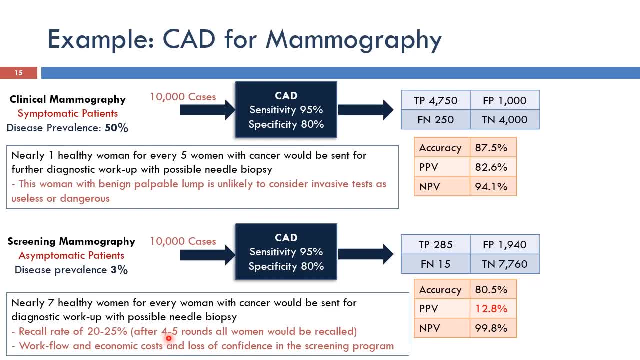 And this is basically a very large percentage. For example, if you have, after four or five rounds, almost every woman will have to be recalled, basically. So, basically for every woman, every normal woman, every healthy woman, she would have to do testing every five years. 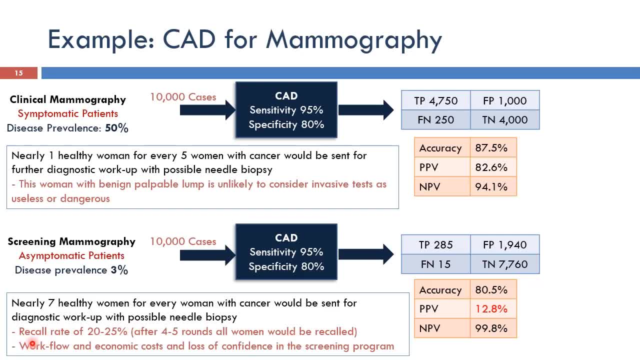 for the testing, which is really unnecessary. okay. This poses workflow problems, economic costs and loss of confidence in the screening program. If the woman goes to the screening program and knows that the results would really come positive most of the time, without being correctly so, 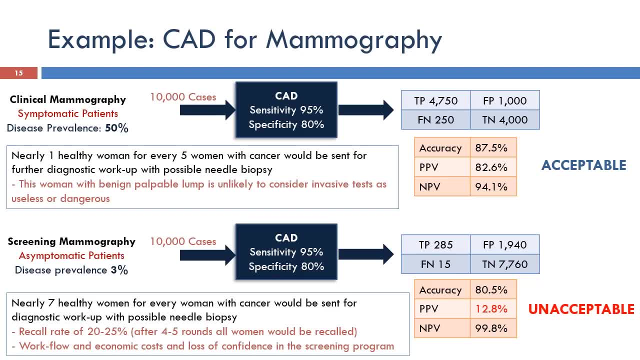 so basically this would be a big problem. So basically in this case we can consider the first one here, the condition here, the same system here applied to clinical mammography, to be very acceptable. The same system, the same CAT system. 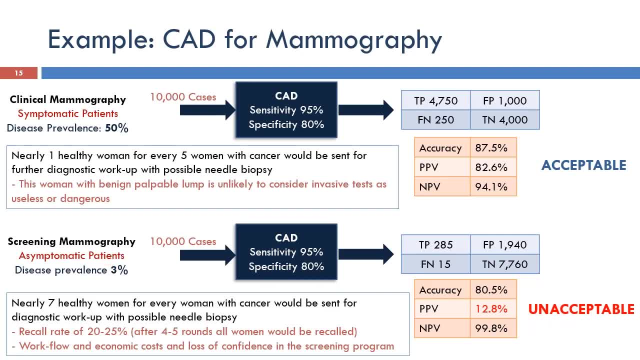 applied to screening mammography would be unacceptable. So there are things beyond the design of the system, the CAT system itself or the technical parameters of the CAT system itself, like, for example, disease prevalence, that would affect the acceptability of the system in biomedical engineering. 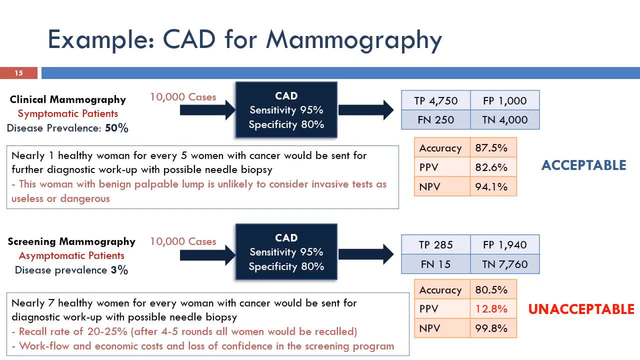 So this has to be taken into consideration. If you're going to develop a CAT system, a computer diagnosis system for a particular application or a particular area, even okay, you have to actually study the disease prevalence in this area and you have to adjust the design of your system. 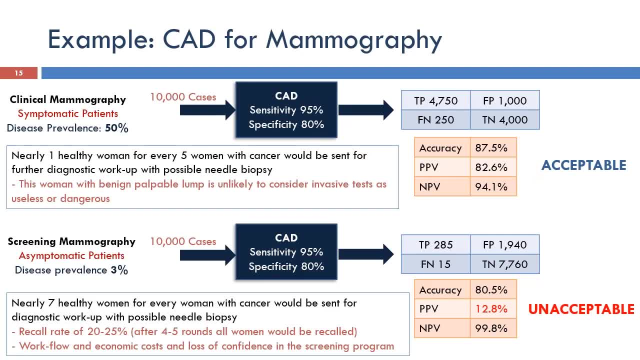 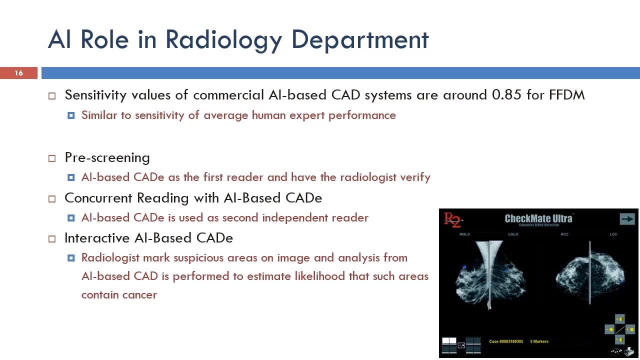 so that the sensitivity and specificity would provide acceptable outcome for that particular application or that particular area. This shows the importance of local development of AI systems, not just getting AI systems that are basically one size fits all, as you see. So the AI systems can serve basically in different areas. 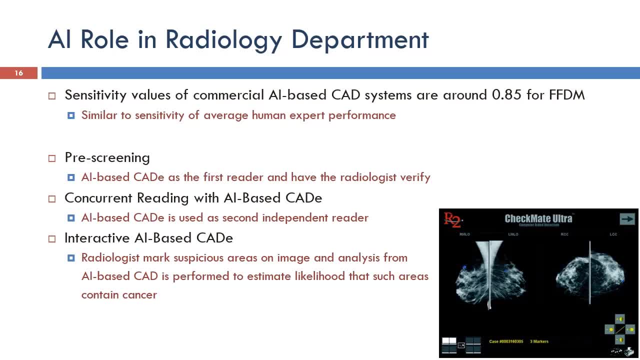 in the radiology Right now, the commercial systems of CAT. you know they have about basic sensitivity of about 85% And basically this is very close or a little bit higher than the average radiographer And so basically you can consider it. 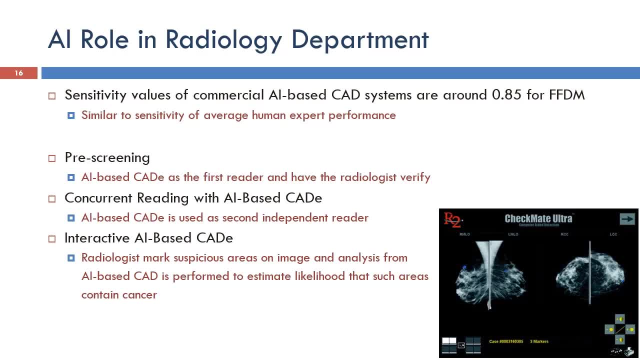 as a second reader. basically, It can be used in different ways. It can be used as pre-screening, where basically the CAT system would basically go over the images and outline the areas that the doctor might need to look at, the suspicious areas. 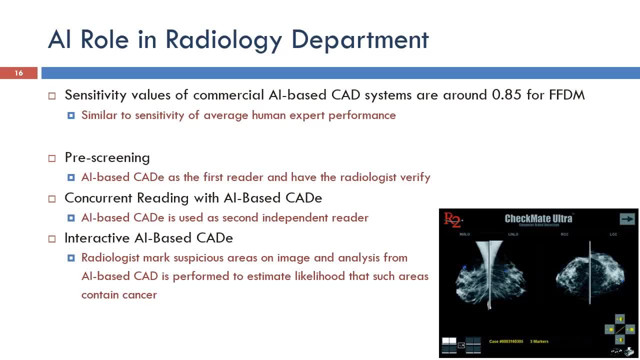 Okay. so basically it would make the life of the radiologist a little bit easier. It can serve as a concurrent reader. So basically, for the pre-screening, the doctor starts from the outcome of the AI system or the CAT system. 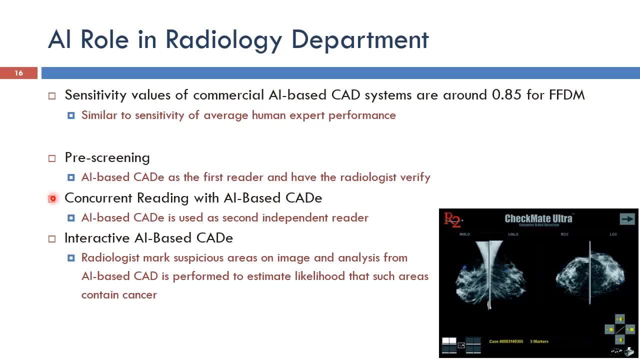 Here. no, it's basically the work in parallel. You don't see what each others are doing And basically at the end you try to reconcile the reports from both. Okay, so basically in this case it can work as a second independent reader. 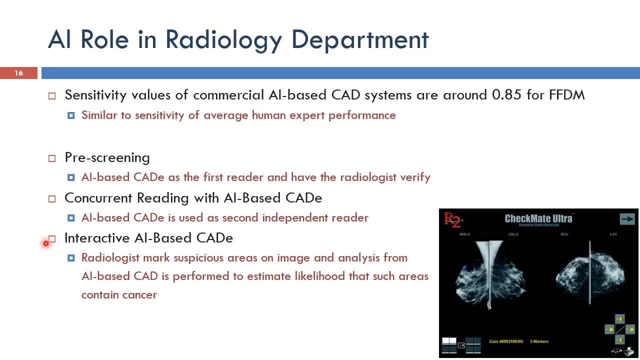 Or it can be used as an interactive AI-based CAT system where basically the doctor would outline the area where he's suspicious about and then the CAT system would analyze and give him a percentage of or a probability of, basically the results. So basically this area being cancer and basically makes 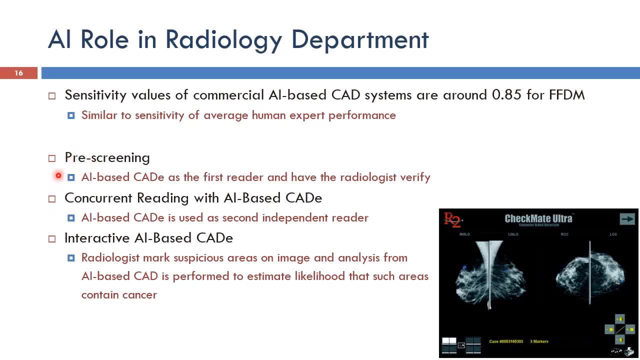 his decision at the end based on that. Which one of these can be used or which one of these is better is a subject of debate between doctors or the medical community in general, But actually at least they are there And basically we can choose one of them. 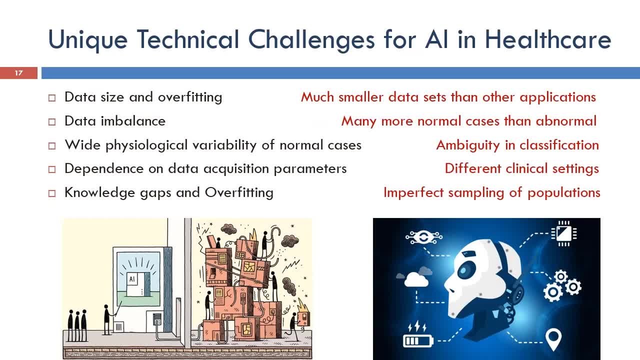 for a particular application that would best suit that particular application. There are several unique challenges for AI in healthcare and biomedical engineering in general. The first one, as we saw, is the data size and overfitting. We have much more data sets than other applications. 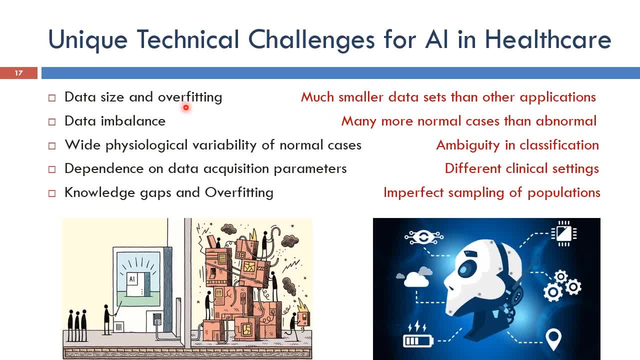 and this basically would cause a problem of overfitting. So basically, we have to start thinking about data augmentation techniques or try to basically advance the field of data augmentation in order for us to solve this problem. in biomedical engineering, We have the big problem in data imbalance. 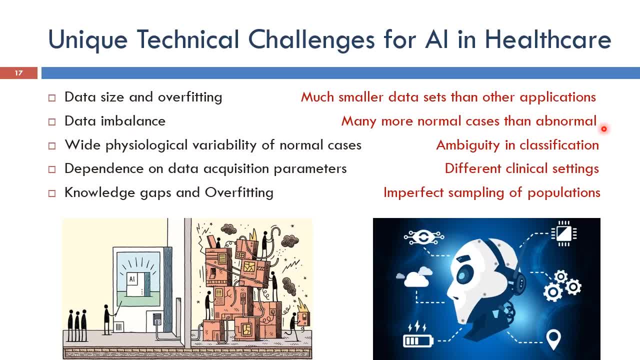 There are many more normal cases that are normal. Alhamdulillah, we don't have as many disease cases as the normals. So basically, this is a good thing in general, but actually for AI systems this is a big problem. 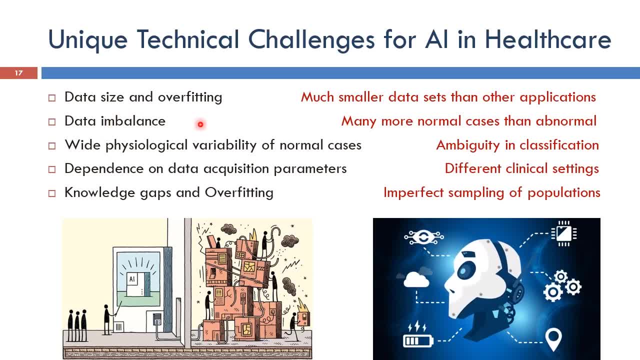 Because whenever you have data imbalance in your input, then the design of the AI system would actually be biased towards the class that has the most data. You also have wide physiological variability of normal cases, which basically makes the normal class very wide actually. 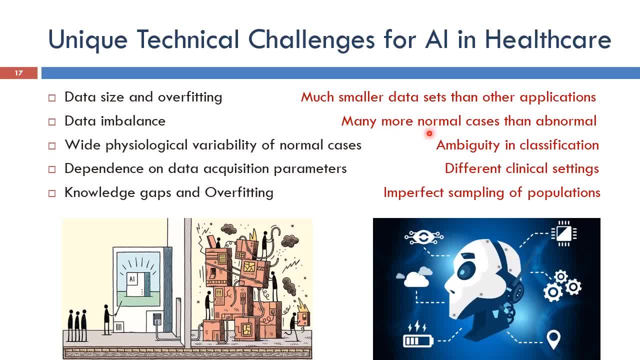 It can actually look like multiple classes, not just one class, which basically causes ambiguity in the classification part. You have also a big problem in the dependence on data acquisition parameters. If you consider, for example, ultrasound imaging or MRI, you have so many different parameters that can be used. 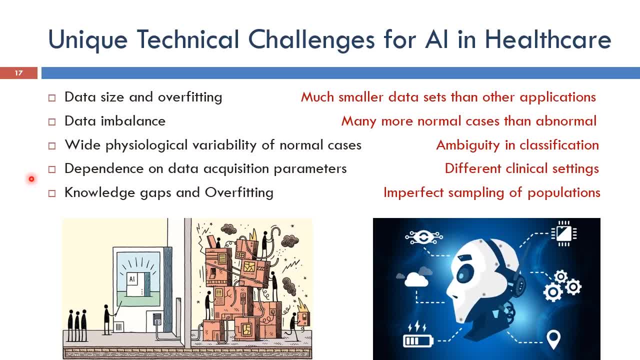 and depending on these parameters, the images would look very different. For example, in MRI you have, basically you have at least four different contrasts in MRI And basically these four contrasts would provide for the same patient for the same location. 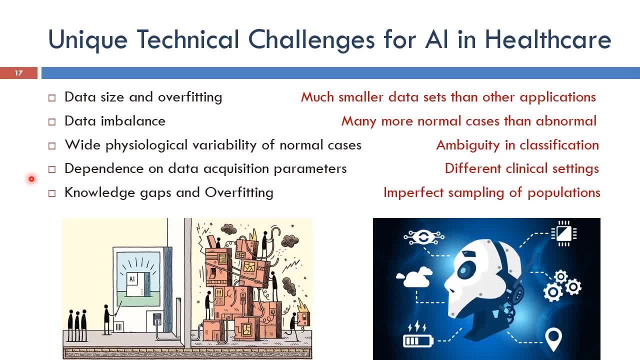 very different images, And so if you want to have a particular AI system trained on these data, it's going to be extremely difficult. You have to basically choose a very particular way of acquisition or standard acquisition parameters, And basically use these acquisition parameters. 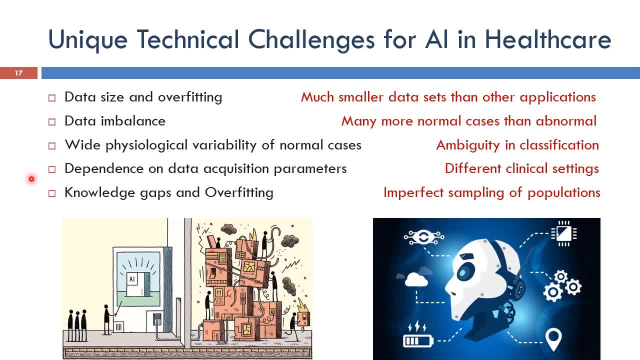 whenever you are trying to use images for the AI system. Okay, So this is a big problem. You have definitely knowledge gaps and overfitting, which results from imperfect sampling of the populations. Basically, sometimes you have very few cases. Basically, it's related to data imbalance. 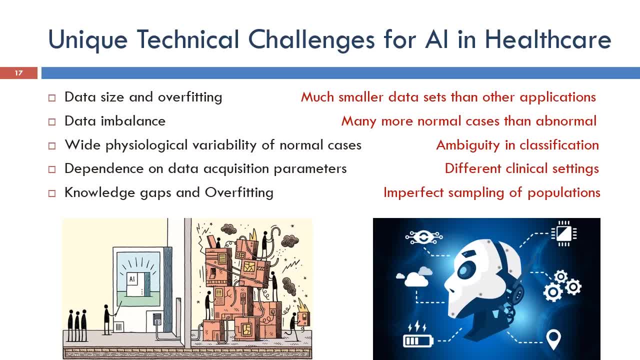 but actually this is a little bit related to the disease prevalence, for example, And basically this can happen- you know happened- in communities where they don't have any- you know enough samples for a particular disease. So basically, whenever it comes, 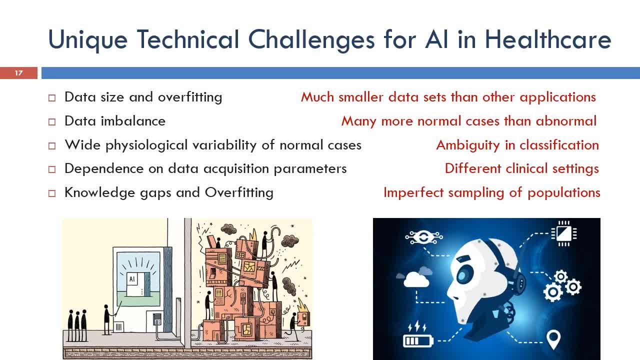 or whenever a new disease comes, it becomes difficult for the AI to identify it. So basically, this is a big problem We don't really have in medical community in general or the biomedical engineering applications in general. it's very difficult to do perfect sampling of populations. 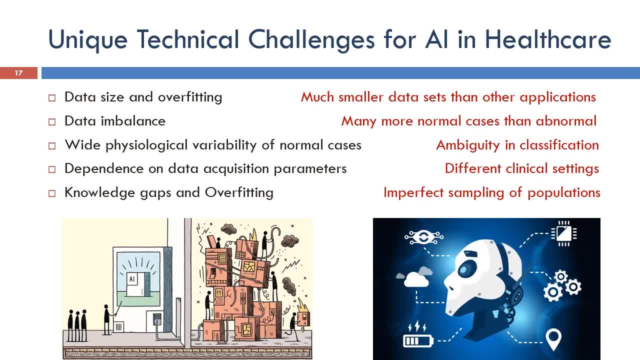 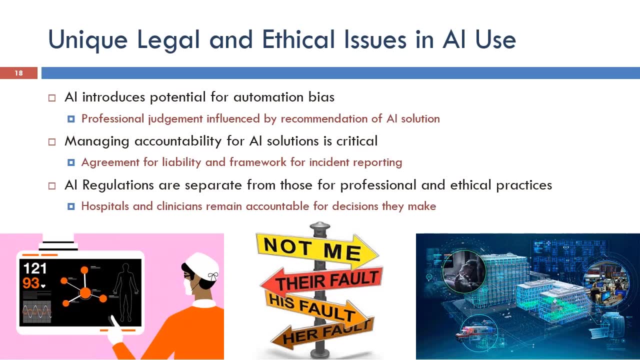 Okay, The population are not uniform, so they are not, you know, even accessible to us sometimes. So, basically, it's sometimes difficult to do the perfect samples that would be required to build a useful AI system. There are also unique legal and ethical issues in AI use. 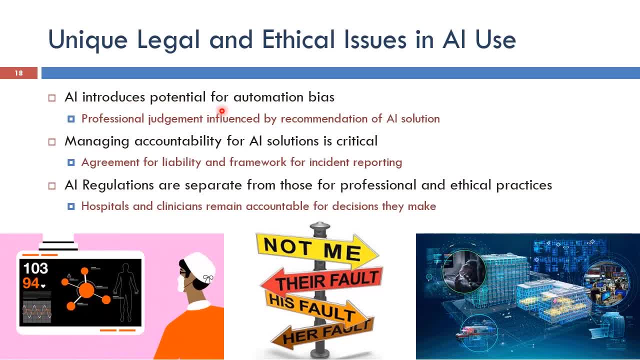 Okay, The first one is basically that AI introduces potential for automation bias where the professional judgment can be influenced by recommendation of AI solutions. When we said that the application of AI can be as pre-reading- okay, Basically, this can be actually a problematic thing. 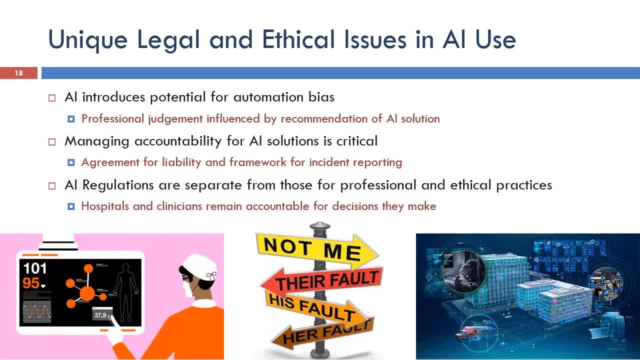 if the doctor would consider the AI outcome as basically something that has a confidence, basically if he has confidence in the system beyond his own expertise, then it can be a problem. So this is a real problem in medical diagnosis, where the doctor can actually be influenced. 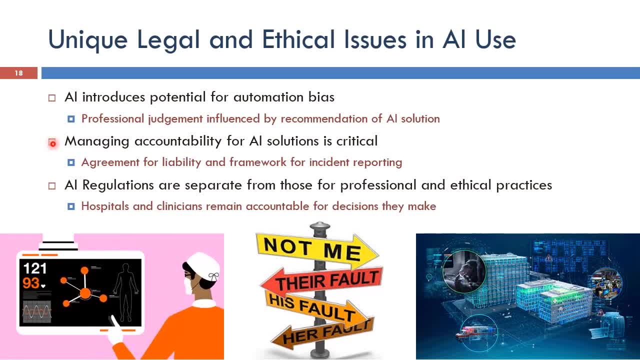 by the outcome of an AI system. Another big problem in the medical applications is that you have to manage accountability. Okay, Meaning that, who is accountable for the outcomes of the AI system? Okay, You have to have an agreement for the liability and framework for incident reporting. 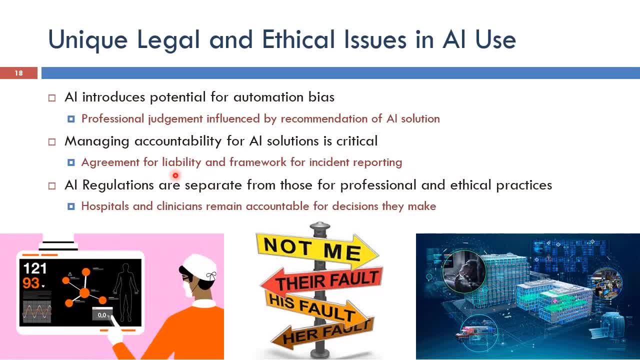 So liability meaning that if the AI outcome was incorrect, who's going to pay for the? basically, if you have a liability for the AI outcome, who is going to pay for the? basically, if you have a liability for the patient, if you cause damage to the patient, 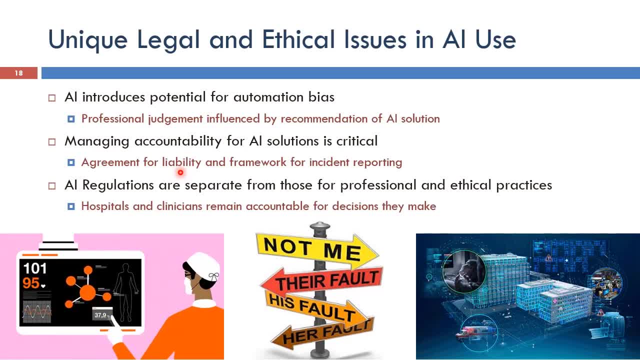 and the patient filed a lawsuit and basically the hospital might be fined or basically somebody has to be responsible for the damages that occur to the patient. So basically there should be an agreement between whoever develops an AI system and the place where the AI system would be applied. 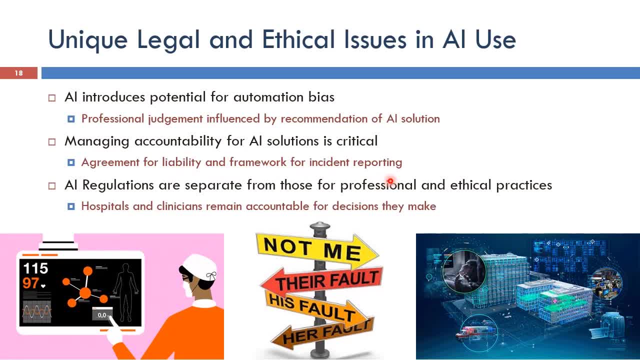 so that this liability can be very clear, And also whenever an incident happens, whenever a situation where actually an incorrect diagnosis caused harm or basically an incorrect diagnosis was discovered, there should be a framework for incident reporting so that these kinds of incidents can later on use to improve the outcome of the AI system. 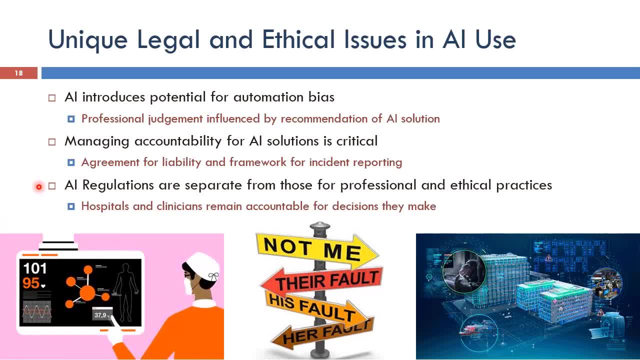 And we have to also emphasize that AI regulations are separate from those of professional or ethical practices, meaning that, basically, if the doctor decides to use an AI system, regardless of the outcome of the AI system, okay, he's still accountable because basically he's the responsible professional. 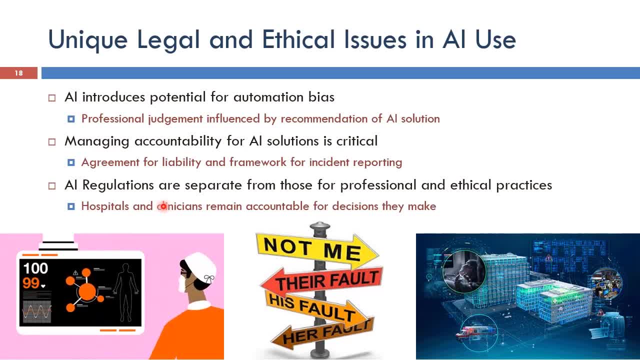 who is in charge of a particular patient. So, basically, the hospital and the clinicians are still accountable for the decision they make, including the use of AI. So this is extremely important to be kept in mind, because the doctor cannot say that it's basically. 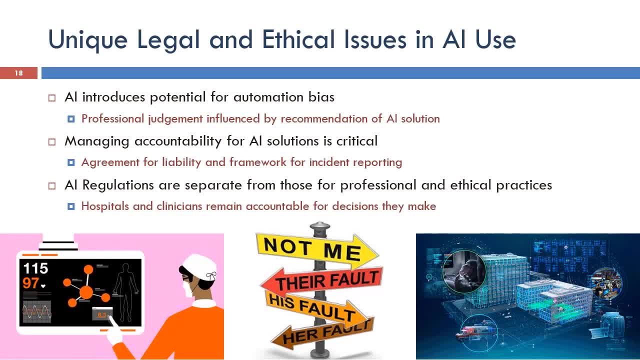 it's the AI system that says so and I have nothing to do with it. It's not like that. Basically, it's his decision. at the end, We developed AI systems that are assistant to the doctor. They are not replacing the doctors. 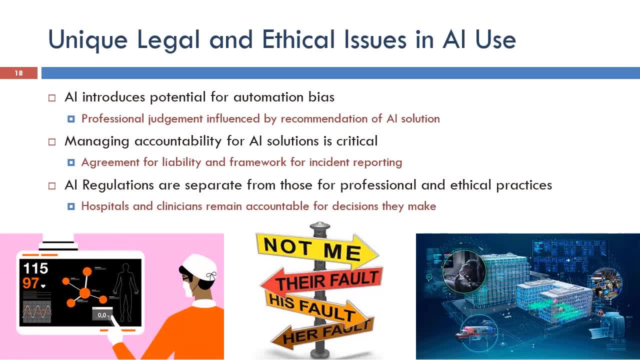 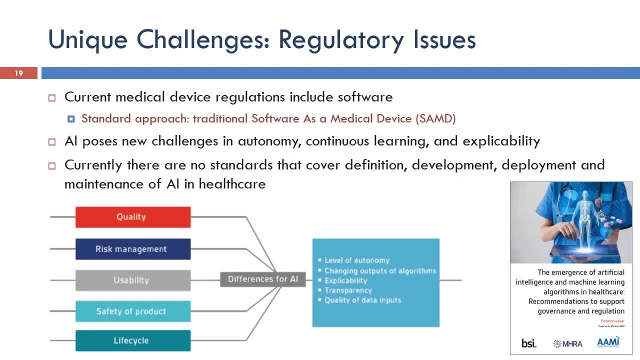 So, basically, it's the decision of the doctor at the end and it's the accountability that lies on the doctor and the hospital at the end. There are also some unique challenges on the regulatory side. We're talking now about somebody who developed an AI system. 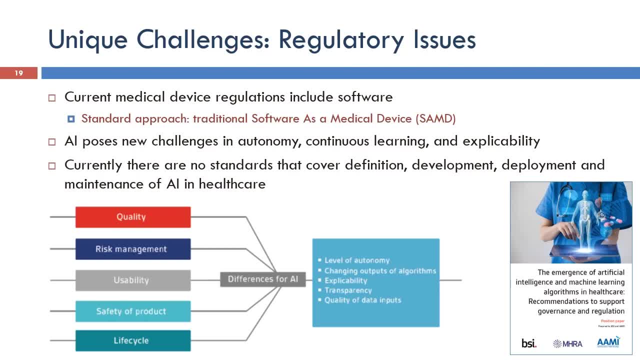 and wants to basically push it into the market, push it as a product. In order for us to have a medical software, we have to actually get an approval from. for example, here we have the Saudi FDA. In the US it's the FDA. 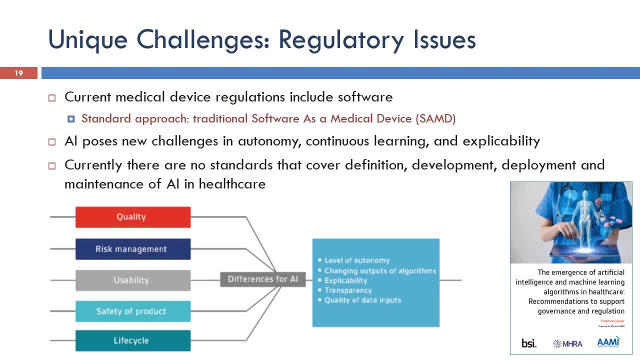 In Europe you have to have CE mark or CE approval. Right now, the way the regulation of such data, such devices, happen is very much like what they do with hardware devices. So basically the standard approach is called software as a medical device, SAMD. 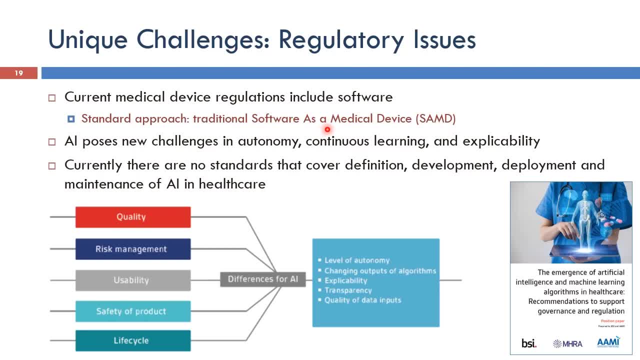 So basically they apply almost the same standards for medical devices. the hardware medical devices to the software. AI definitely has new challenges compared to the regular devices. basically, You have a problem in autonomy, Basically being working on its own, making a decision on its own, continuous learning. 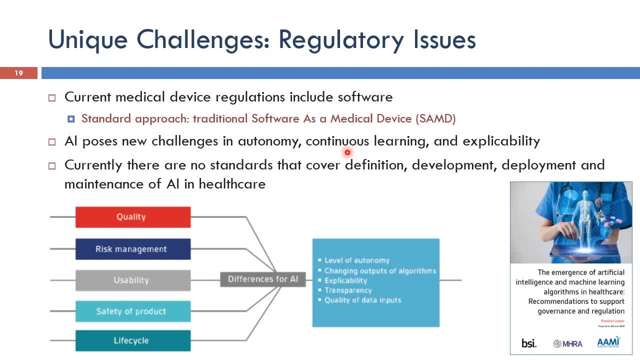 Sometimes, actually, you allow the AI system to continuously learn while it's at its site, So basically, it's an issue that wasn't there before. You don't have any medical devices that continuously learn after you install them And you have a problem with executability, basically, 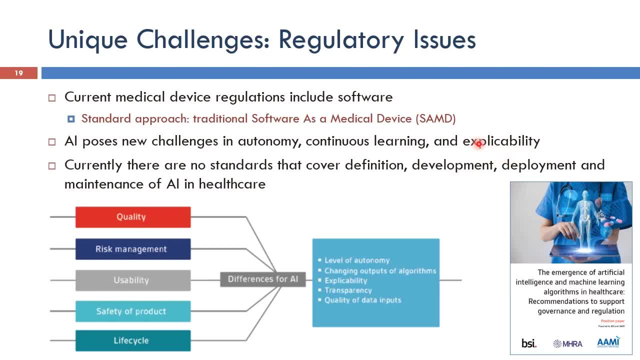 Basically, you have to explain the outcome basically. Basically, you have to explain the outcome, basically, How you came up with this outcome. If you made a wrong decision or make a wrong diagnosis, for example, can you explain why This is a big problem actually? 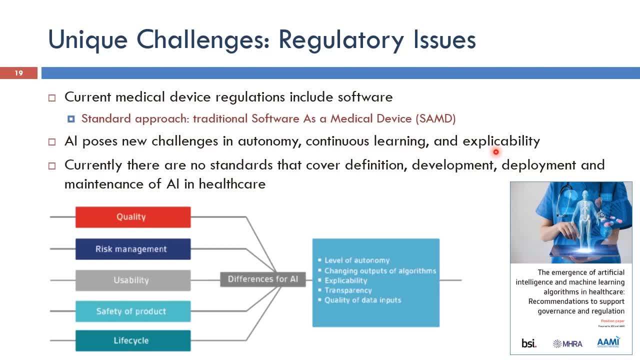 For such intelligent systems like deep learning, for example, it's extremely difficult to get an explainable system. So, basically, you have to actually start thinking about these things in order for- And these things actually, we don't have a solution. 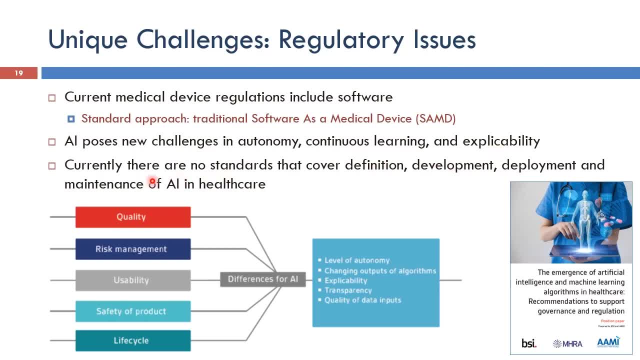 actually, as far as regulation of such things, Okay, So At this time we have no standards that cover the definition, the development, deployment and maintenance of AI in healthcare. So basically we're using standards that were applied for other applications. 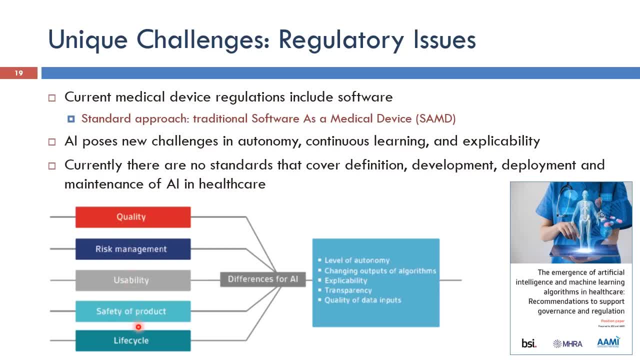 You basically look at, for example, quality, risk management, usability, safety, life cycle, things of that sort that apply to every medical device, But for AI, you have unique challenges that should be actually addressed in a unique standard. This is not here yet. 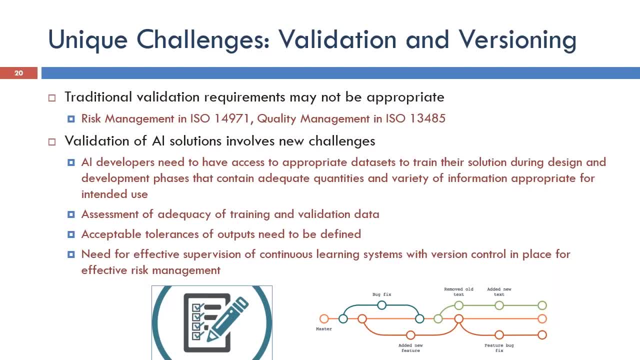 Okay. There are other unique challenges related to validation and versioning. For example, if you're trying to test a particular medical device to be safe, you have certain standards, like the ISO 14971, the quality management for a manufacturer, like 13485,. 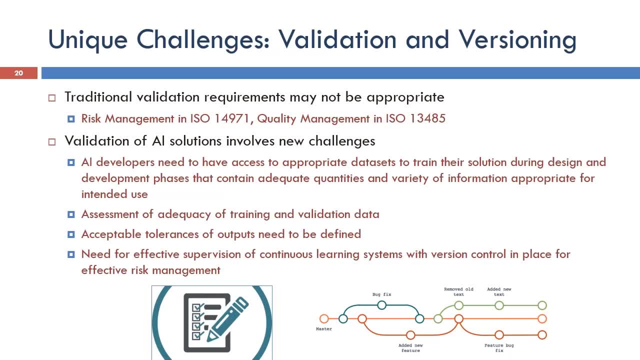 ISO 13485.. And basically they are very much. If you follow these, it's very straightforward. basically, The problem for AI solutions is that it's not as simple. You can apply definitely risk management in AI solutions, Definitely. 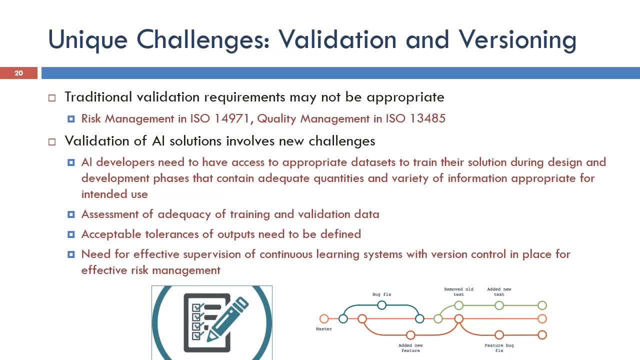 But actually how you're going to apply it is very different. Okay, One of the unique differences is that if you develop your own system, you develop based on your own data, And usually your own data is basically the soul of your product. 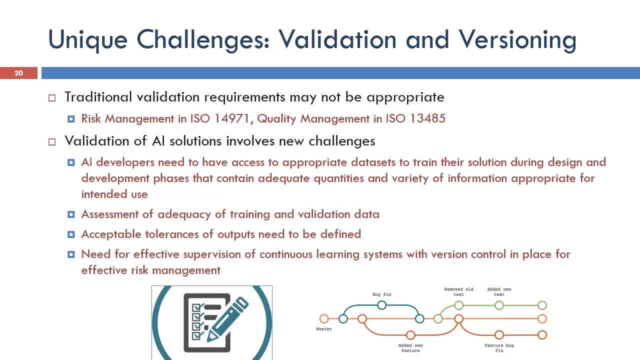 This is basically the know-how of your product. If somebody else gains access to your data, then he might actually develop a better solution okay than yours Okay. So basically, your system is as good as the data you have. So when you present your system to the regulatory agency, 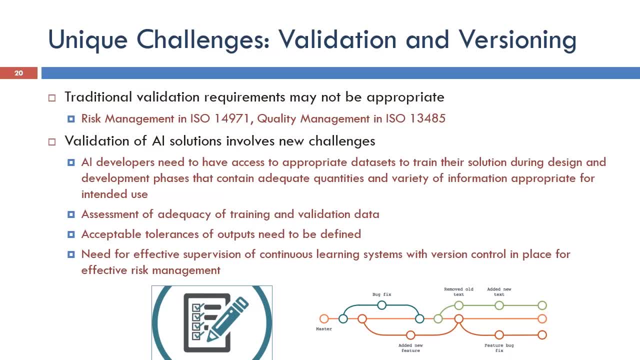 you cannot present the data, It's actually You're giving your know-how, disclosing your know-how, and basically this can be very dangerous, actually. Okay, So basically, how would a regulatory agency evaluate a ready-made or a product in AI? okay, without having the data. 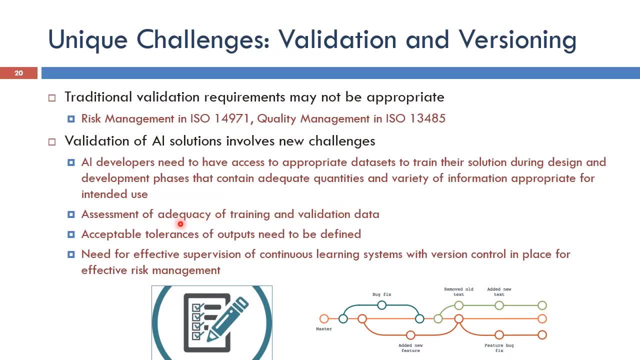 Okay, Basically we have you know. basically, you have to actually discuss the adequacy of the training and validation data used in the development. You can say that we use this number and we got this data from this particular place and it was labeled like this, things of that sort. 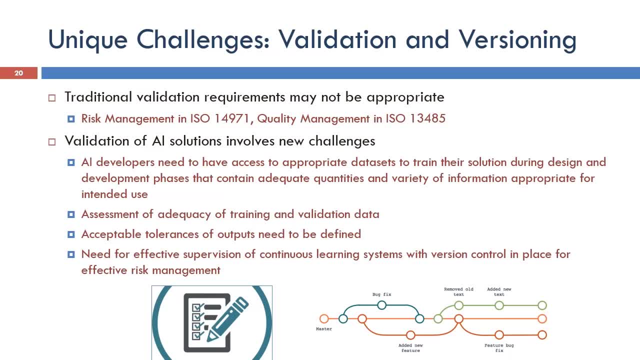 But actually there is no way of confirming that they are actually. you know the way they are And basically, if you want to test it, if you want to test a medical device for electrical safety, there is a device that you can use. 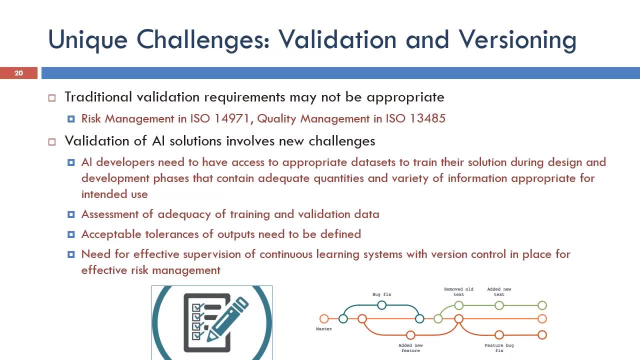 You can apply to the medical device and basically get the measure of whatever parameters you want Here. if you want to test a particular system, would you be able to have your own data set to be able to basically apply the AI solution to the data you have? 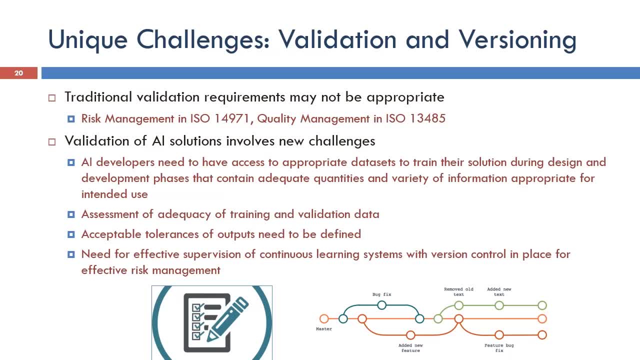 and basically have a uniform way or a coherent way of evaluating different solutions from different manufacturers. This is not really yet sorted out. It's basically people are still thinking how to do that. So basically it's a big problem And definitely there is a bigger problem even for the supervision of continuous learning systems. 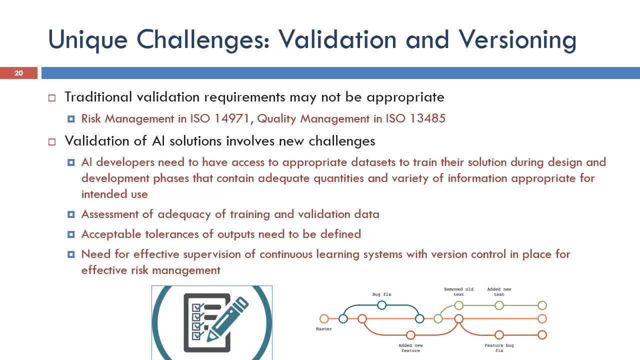 meaning that if you're going to put an AI system somewhere and this AI system would still acquire data and improve itself over time, how are you going to control that? You know, how do you make sure that nobody gave adversarial examples to this CAD system so that it's 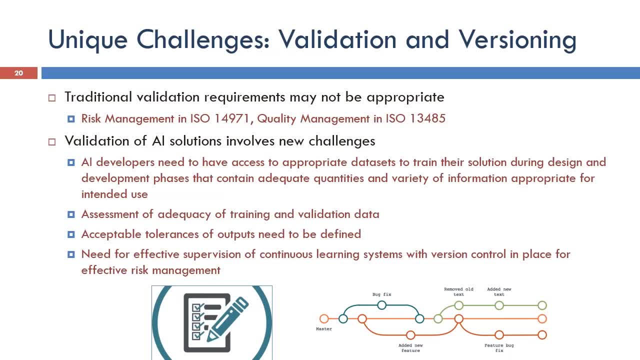 really, really easy to get good results or good results to get good results, And then you have to figure out what is the best way to do this, And a lot of these things are complicated. I'm going to go through the key things and then I'll tell you what you can do for yourself. 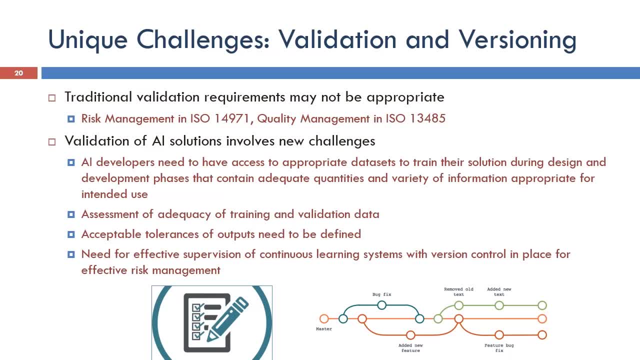 We have to start with the first thing And in the case of AI systems, as I said before, they can be awesome. So what do we have to be able to do? You start with a training and you start with ameasuring it down to an AI product. 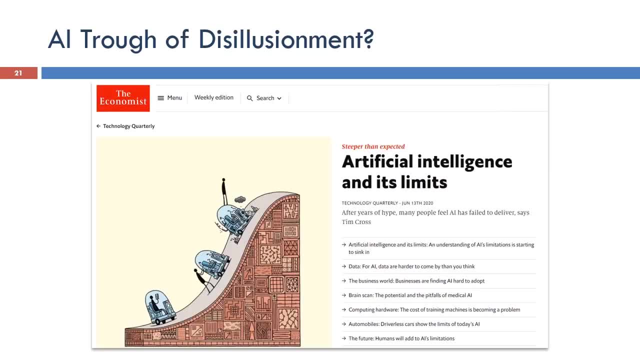 You have to be able to do it in a way that is consistent with the activities that you're doing and specificities that you're doing. You have to teach there and the ways that you're doing things. You have to be able to tell people who can do things. 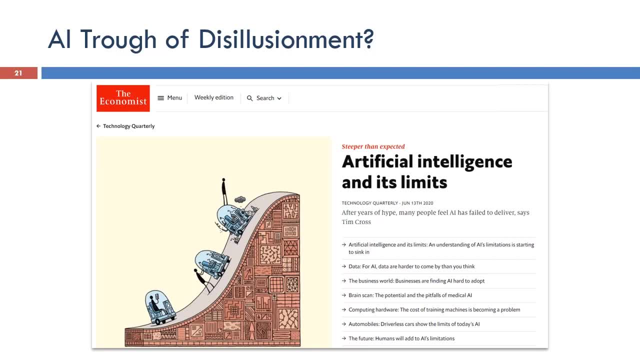 You have to be able to tell people who can do it. i just want to point out that, um, basically we have what's called the technology hype curve- people in every technology. whenever a technology comes out, people start thinking that this technology will do everything. after a while, you think that actually it's not doing exactly what. 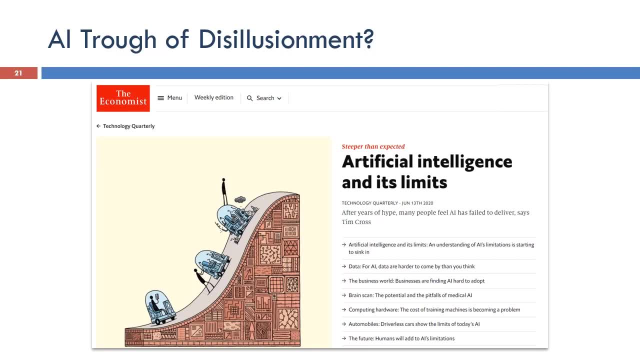 we thought it's actually we. we expected to do this and that and basically didn't do either. okay, so basically, some, some articles actually started coming out, uh, with this kind of statement. after years of hype, many people feel ai has failed to deliver. okay, which is actually, uh, what's called. 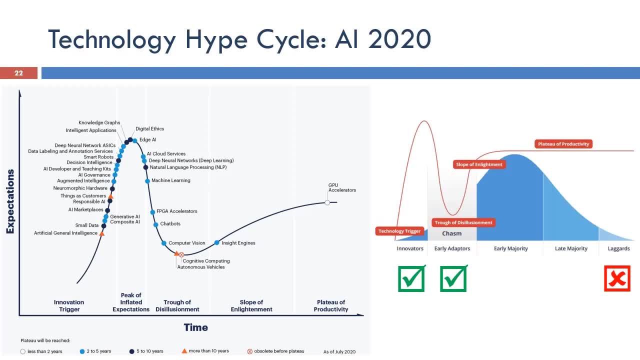 what's basically represented in the technology hype cycle. in every technology, you have something that looks like this: basically, you have the innovation trigger, where the technology actually starts okay, and then the applications, or basically the expectations, soar or basically become really very steep. okay, at this stage, basically, and you end up with: 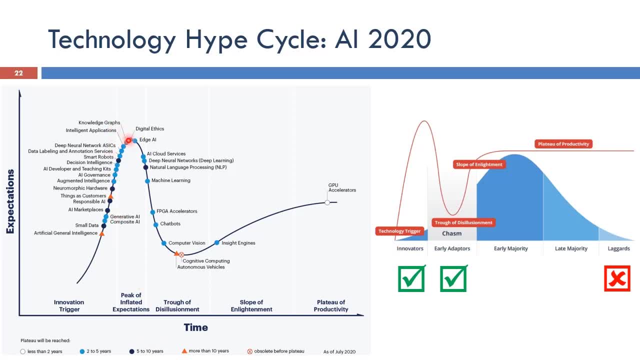 what's called the peak of inflated expectations, meaning that at this point here you have, basically you expect this technology to everything. i saw that before in many applications. basically i saw that for the neural network, the initial neural networks. basically in the early 90s, for example, people expected the simple neural networks to do everything and basically 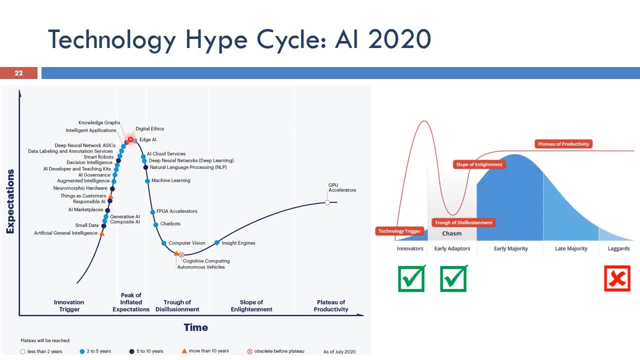 they ended up a few years later to be very abandoned. basically they were abandoned for a few years and then deep learning basically pushed it back, basically when the technology of deep learning that basically, uh, revived the neural network technologies. basically i saw that with wavelets, for example- okay, people also will. when wavelets came out, they thought: 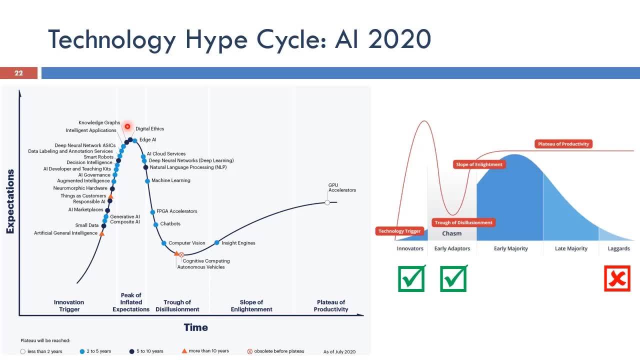 wavelets will actually do a lot of things or basically do, uh, most of the things that people would want to do in signal processing, for example, but actually now they are basically not like that. basically, people realize that you have to have realistic expectations. unfortunately, whenever you have inflated expectations and the technology fails, 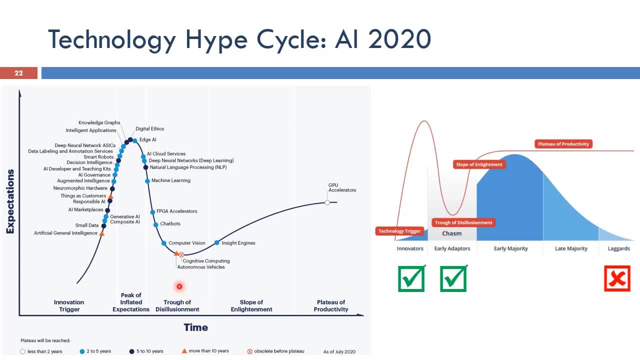 to deliver, then you're basically end up in a what's called trough of disillusionment. you're disappointed, really, of the technology and at this point here you think that the technology will not do anything. basically, it's a failed technology. we should abandon it. but this is incorrect. actually, the right thing to do is basically start thinking about the. 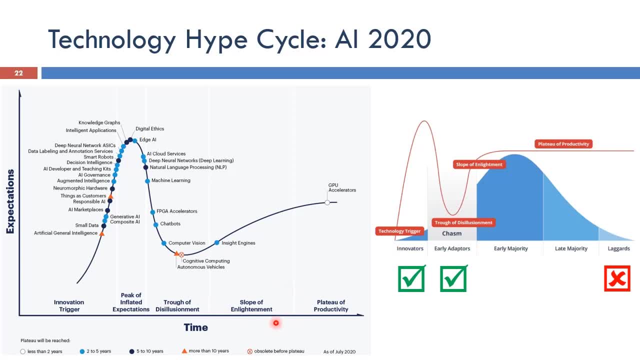 technology with realistic expectations. so basically we have here what's called slope of enlightenment. enlightenment meaning that you start basically looking at the the pros and cons of the technology and slowly but surely actually reach something called the plateau of productivity. here you basically you're talking about the realistic expectations. 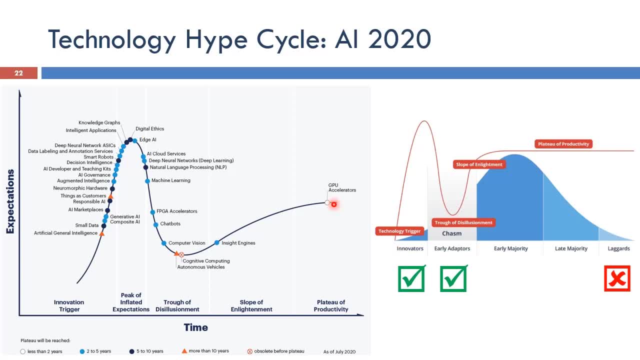 that can be delivered. okay, this: this is the stage where you have products out of whatever technology that you have. this is the hype cycle for 2020. as you see here, neural network, deep neural networks- are basically slipping out of the peak of infinite expectation. they are right here, right. 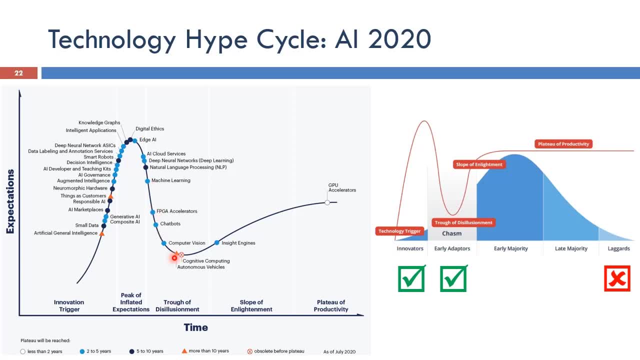 now, okay, machine learning starts slipping a little bit more. okay, so basically they are coming here very soon, basically. but we know that these things are very useful, they have a very good application, but they are not the universal applications or the perfect performance that we expected when we were here, for example. okay, so basically we should start right away to basically 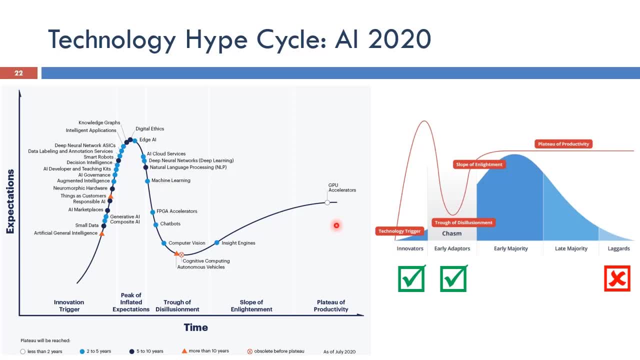 try to understand the limitations of each one of these and try to have realistic expectations so that we can end up in the plateau of productivity very soon. usually it's better for us to work here in these two areas. basically, we have a lot of applications and we have a lot of applications. 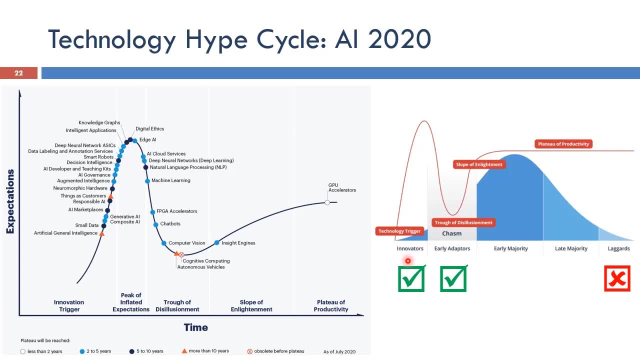 and we have to have what's called the early part here, which is the innovators part, where people can actually shape the technology. uh, here we're talking about the, the slope of enlightenment, we talk about early adapters. early adapters are the people, uh, who actually realize the potential of 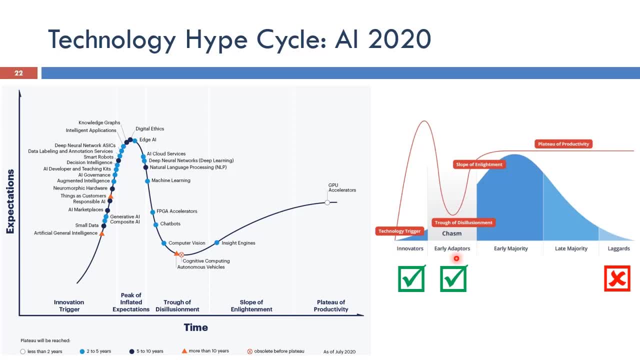 the technology and also the limitations, and basically started doing actual production or actual product development using that technology. okay, so basically, this is also very good. if you catch on with the technology, you're going to have a lot of opportunities and you're going to have a lot of opportunities. 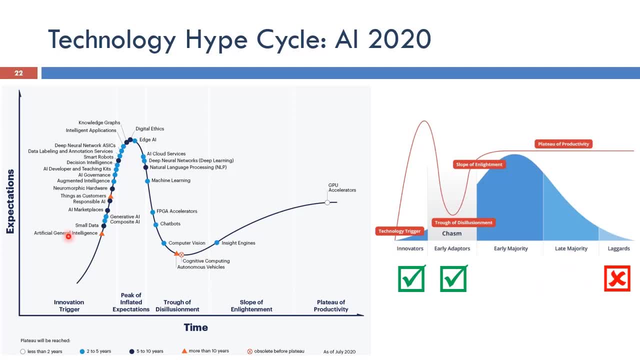 but you don't want to spend time��세요zem the technology a little bit later than you basically missed out on this technology. you probably wait for the next technology then, okay, so basically it's better to uh whenever a technology comes out. we, we don't just think about the potential, we. 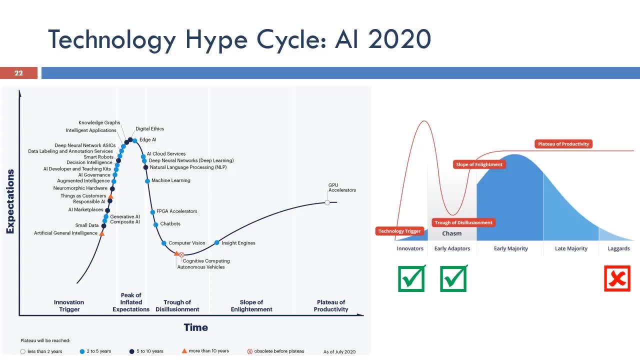 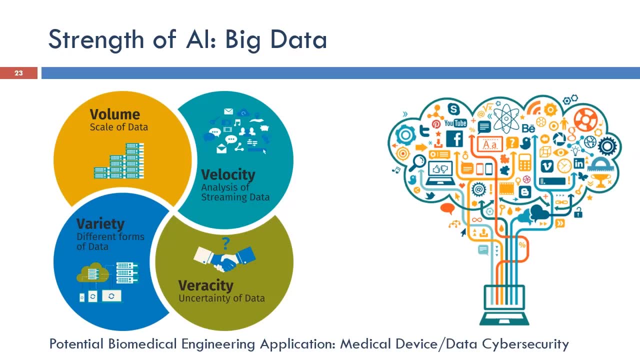 think about also the limitations so that we can get started right away, you know, in product development, rather than hyped expectations. one of the best applications of ai that i actually seen by medical engineering is uh, in the, And they're biomedical data cybersecurity, basically For the cybersecurity. we heard during the pandemic actually that many healthcare facilities were hacked by hackers, basically. 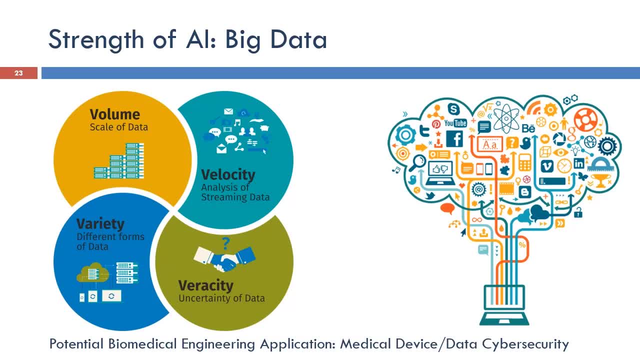 Whether it's ransomware or otherwise, this can be a very big problem And basically now we are using things like PACs, we're using telemedicine things of that sort, So they can be interrupted very easily with a hack. 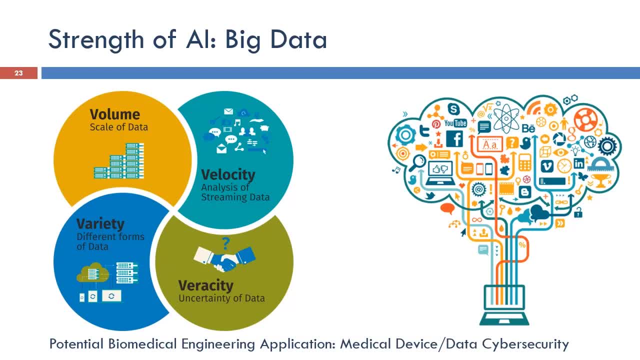 Basically, if you have a computer hack or something like that, it can basically interrupt the services, the medical services, for unknown periods of time And basically can cause harm to patients. Actually, the first patient that died out of a hack was in Germany last year. 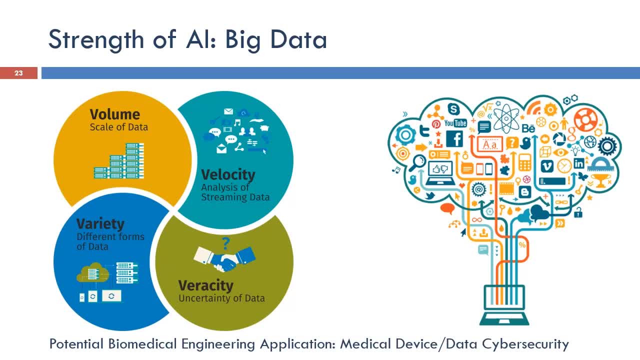 So basically this is dangerous Basically for the data. You know the data that comes in and out of hospitals. these are huge amounts of data. They are literally big data where you have very large volumes, very high velocity. Basically, the streaming data are going at very high rates. 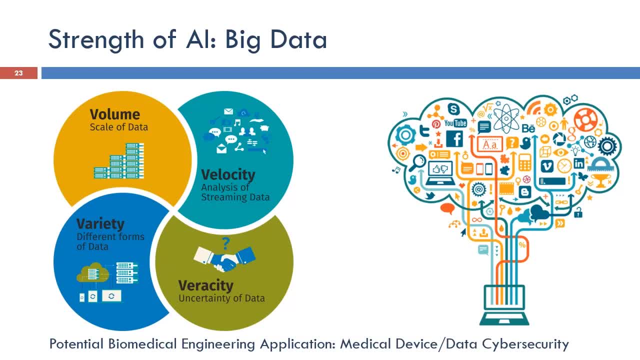 And you have a variety of data. okay, Variety meaning that you have different kinds, You have images, you have signals, you have reports, you have all kinds of things. So, basically, you have the basic definition of big data, is there? 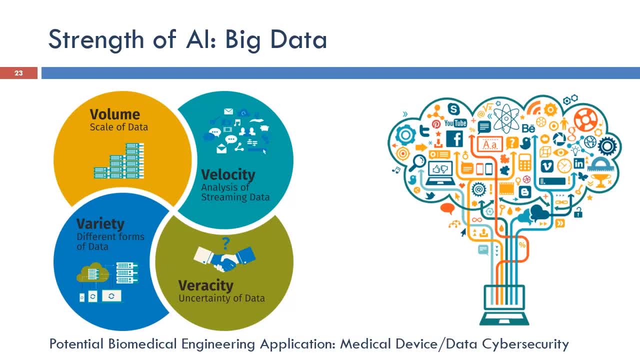 In order for a human being to To observe all of these. it's extremely difficult. AI systems can actually be trained to catch the Or basically be used in defense, cybersecurity, defense mechanisms. okay, And basically this is one of the big applications that I see for AI and biomedical engineering, in addition to the other applications that we talked about. 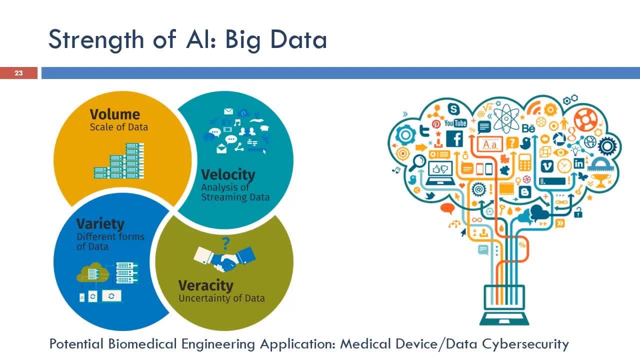 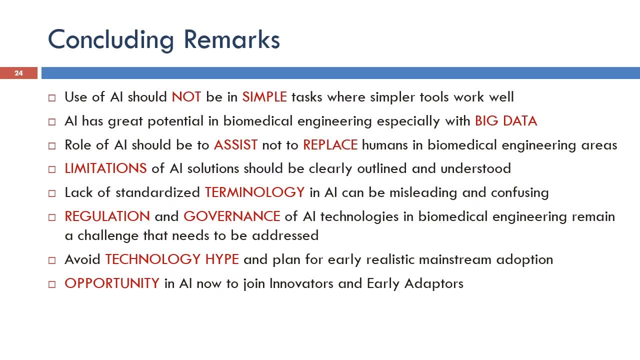 But this actually will catch on and will be very major improvement actually to the cybersecurity of medical facilities. So, in conclusion, the use of AI should not be in simple tasks where simpler tools work well, Because basically it doesn't make sense to use deep learning network with millions of parameters where we can actually do a regression model that has one or two parameters and that's it. 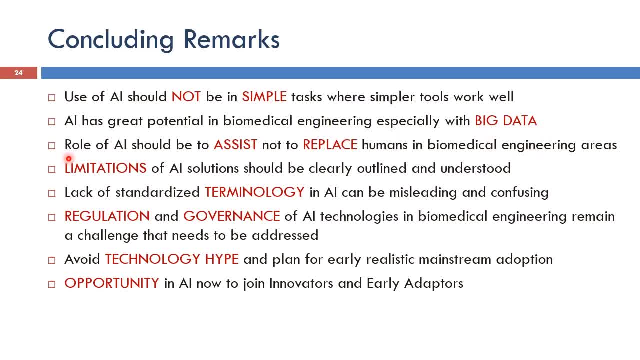 AI has a great potential in biomedical engineering, especially with big data. The role of AI should be to assist, not to replace humans in biomedical engineering. The limitations of AI solutions should be clearly outlined and understood in order for us to actually realize the potential of such solutions. 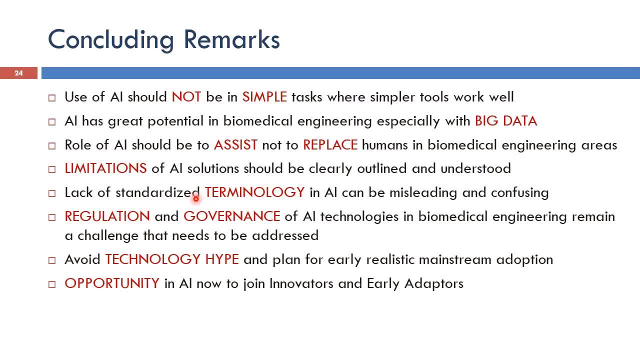 The lack of standardized terminology in AI can be misleading and confusing and should be actually addressed as soon as possible. The regulation and governance of AI technology and biomedical engineering remains. They both remain a challenge that needs to be addressed. Avoid technology heights. Avoid technology heights. 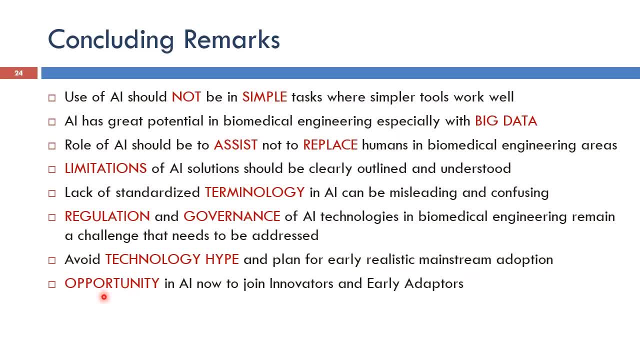 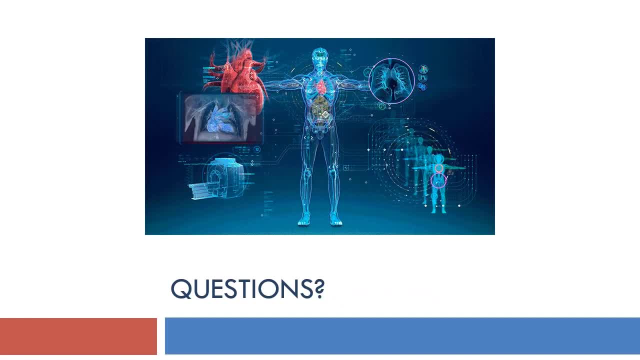 Avoid technology heights And plan early for realistic ministry adoption. And we have an opportunity in AI now to join innovators and early adopters. Thank you very much. 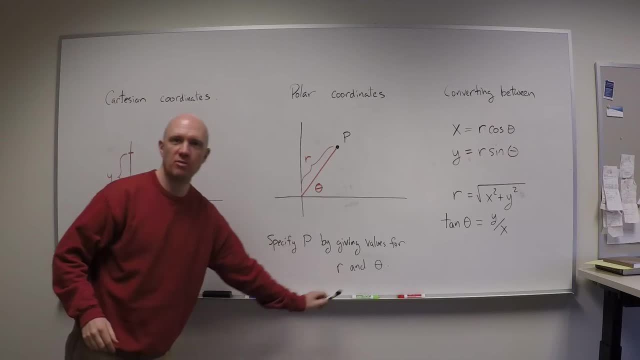 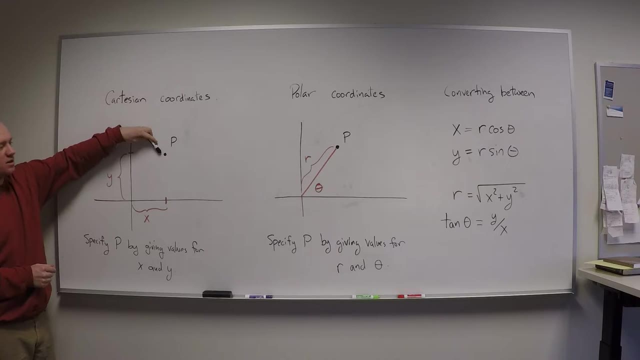 Let's talk about polar coordinates. So you're familiar with Cartesian coordinates. You think about specifying a point in the plane via the Cartesian coordinates by simply saying how far along the x-axis I have to go and how far up the y-axis I have to go, in order. 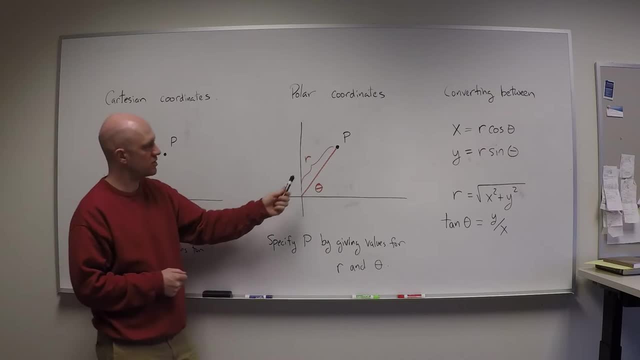 to get to the point. Well, polar coordinates are another way of specifying a point. We keep the x and the y-axis here just for reference, to kind of see where we are. And this time, instead of saying, oh, I have to go over x and up y, I say that I have to go through. 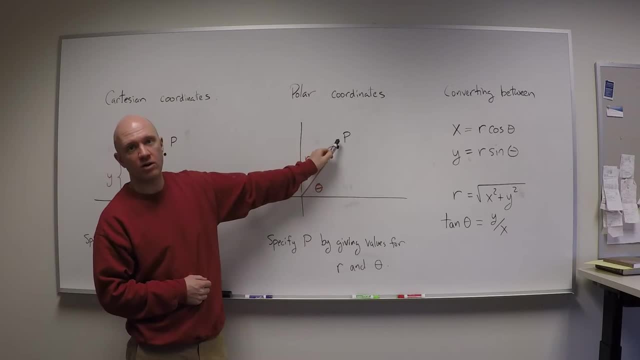 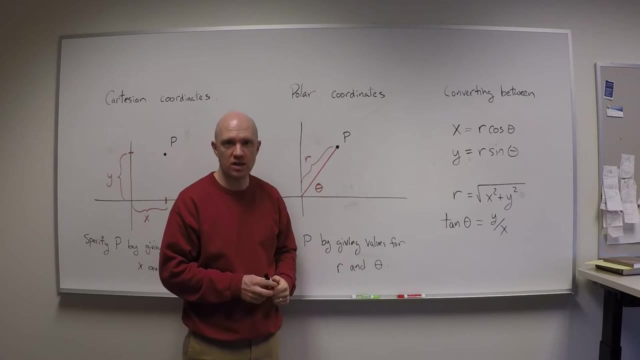 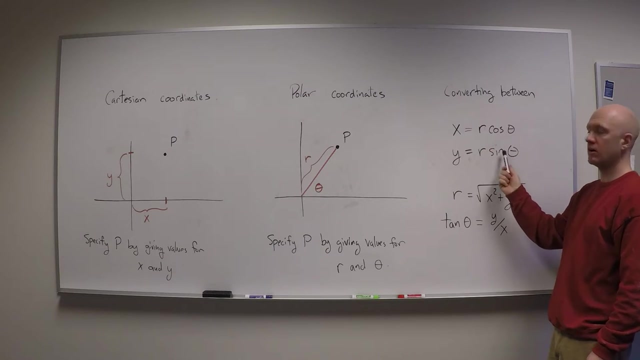 an angle of theta and then out a distance of r from the origin, And so we can get between Cartesian and polar coordinates using some trig. So for example, we have this conversion that says: if I know what r and theta are, I can then tell you what x and y are, And 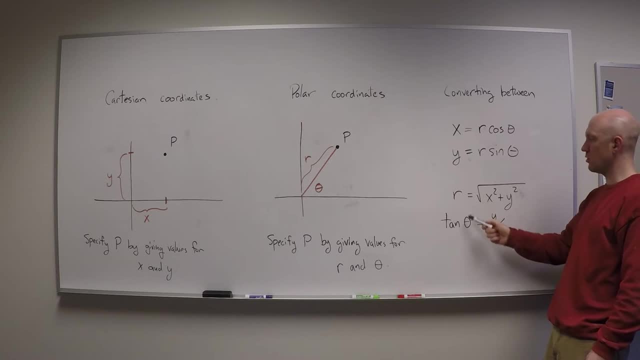